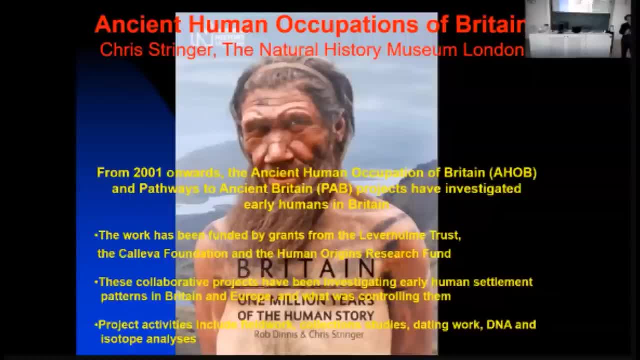 the big papers in our field, And so he is able to keep up with the pace of new scientific results and research. And on the back of social media such as Twitter, he's carved a large following which I would thoroughly recommend any young student or early career researcher. 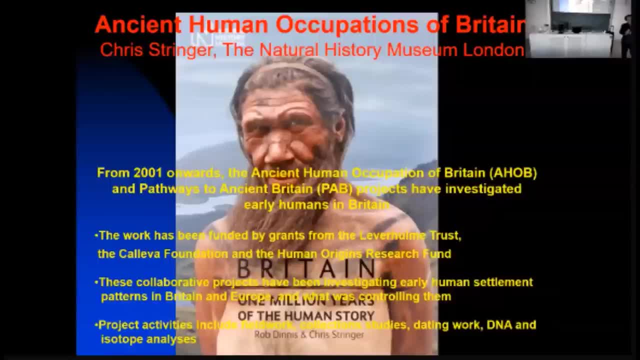 to follow. His career is a long one, and I think it's really important for him to be able to do that, And I think it's really important for him to be able to do that, And I think he's really important for him to be able to do that, And I think it's really important for him to be. 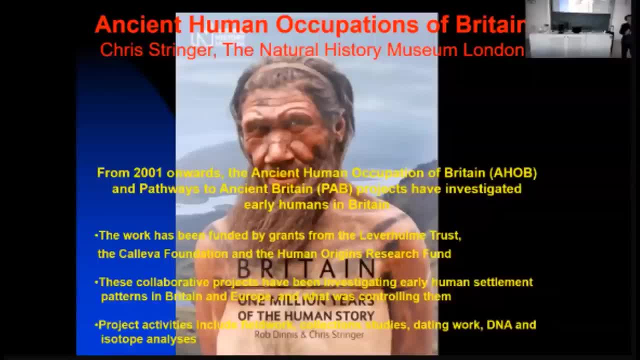 able to do that And I think it's really important for him to take the chance to try. But keeping up with what's happening in our field is something that Chris seems to handle with a plumb, And this stellar career has seen Chris honoured as a fellow of the Royal. 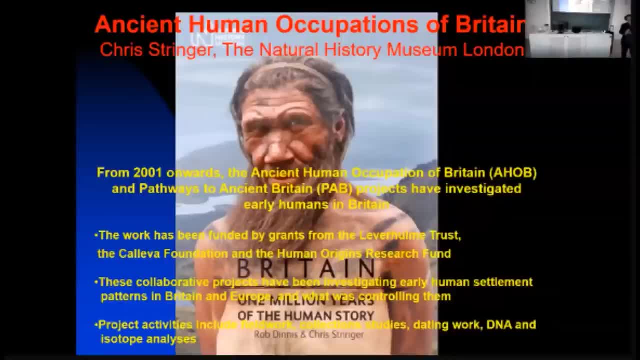 Society and as an honorary Fellow of the Society of Antiquaries, And in addition, he was appointed commander of the Order of the British Empire in the 2023 New Year's Honours List in the UK. the services to understanding human evolution. 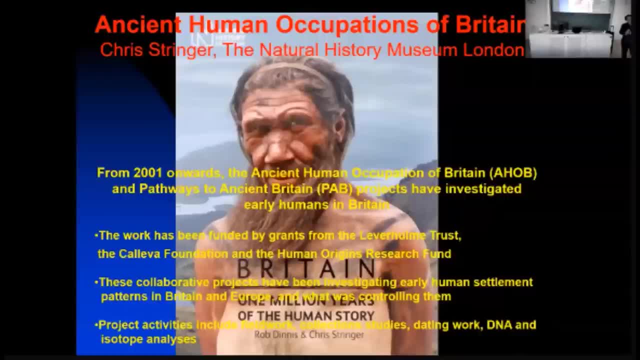 CBEs are awarded to people who are highly distinguished, innovative in their contribution and conspicuous their leading role, something which describes chris very well. tonight, chris's topic will concern the early human occupations of britain, and i anticipate that some of this work will mention the ancient 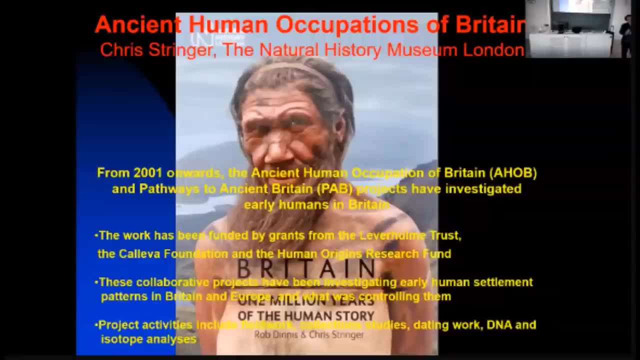 human occupation of britain, or ahob project, which ran for about 10 years from 2001, which chris co directed. this breakthrough consortium project reconstructed and studied the episodic pattern of human colonization of britain during the pleistocene and his follow-up research project. 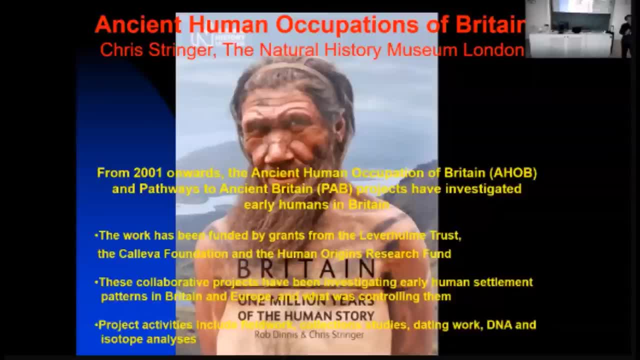 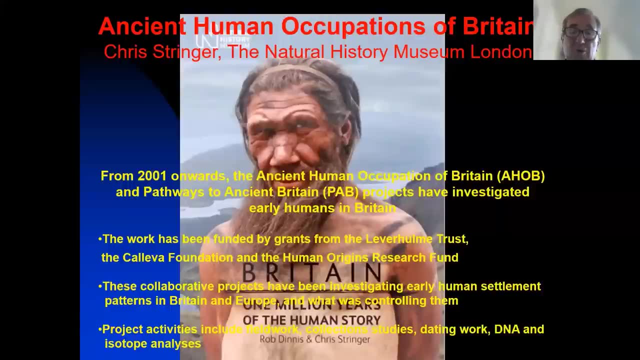 pathways to ancient britain is ongoing. chris, we're really delighted to welcome you here tonight and, without further delay, let's get cracking. thank you very much for that, tom, and so yes, i'm. i'm going to talk mostly about the work of the ancient human occupation of britain, project ahob and the 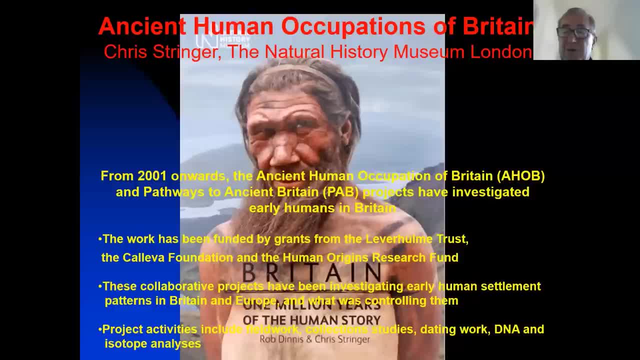 succeeding pathways to ancient britain project. so these projects have been running uh for over 20 years now. ahob was funded by the levium trust and pathways to ancient britain is funded mainly by the kaliva foundation. so these are large projects and they grew larger through time. 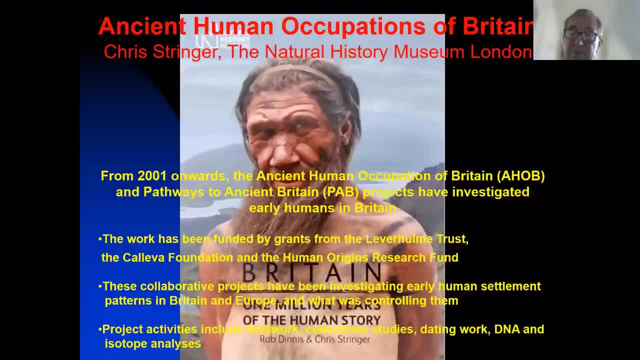 we've have more than 50 members and associate members, and that included tom and katarina, now with you in vienna. so the project activities, uh, included field work, but also a lot of work going back to existing collections, some which had not been properly studied, sometimes for over. 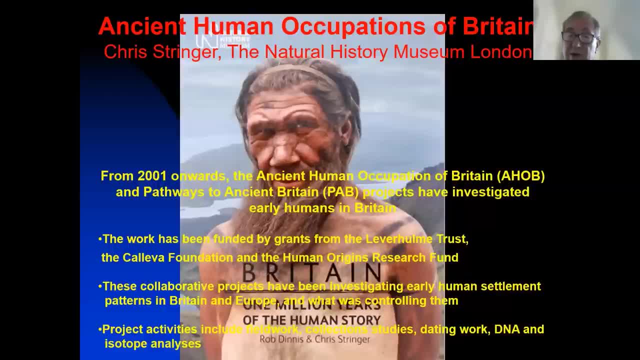 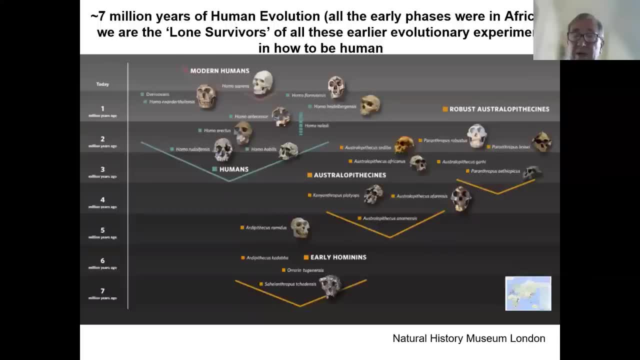 a hundred years and applying things like data analysis and reading work and isotope studies to those collections. so i've got a lot to cover in this time and obviously the bit i'm going to be talking about in human evolution is a very recent bit. so i'm going to be talking about occupations in britain in the last 1 million years or so. so 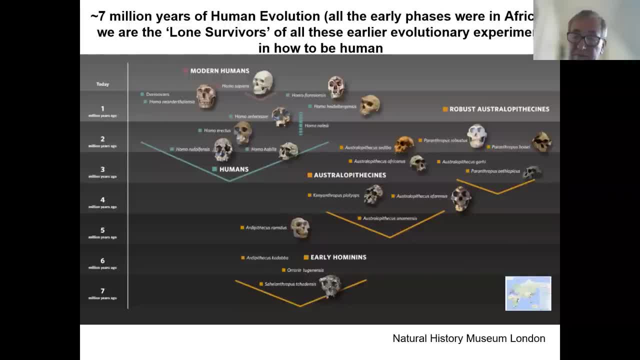 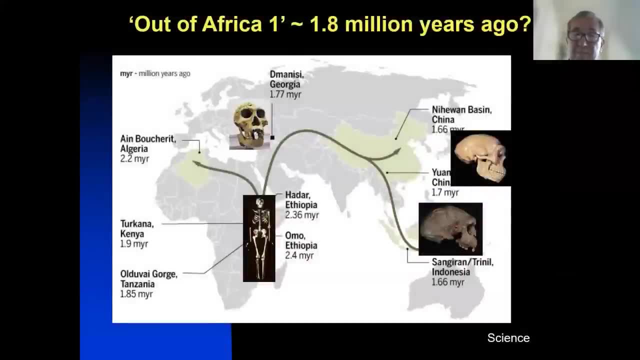 we're talking about. you know the end stages of human evolution, um particularly, of course, our own evolution and that of the neanderthals. so, starting with what's commonly known as outer africa, one um on the conventional view, homo erectus, widely defined, evolved in africa and left there soon after two million years ago. 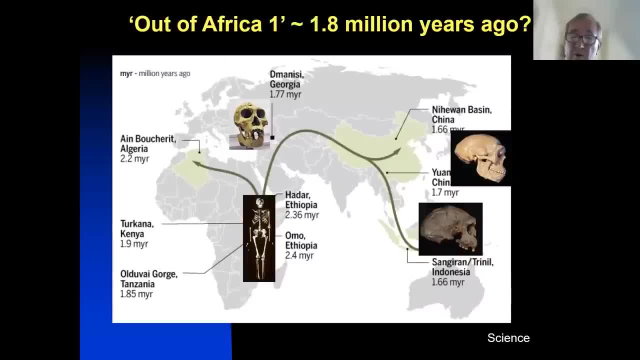 stayed behind as well, of course. and we find humans then in parts of eurasia. we find them over in the far east, in china, in indonesia and java, in dominici, on the fringes close to the edge of the earth, uh, in the caucasus, um about 1.8 million years ago. 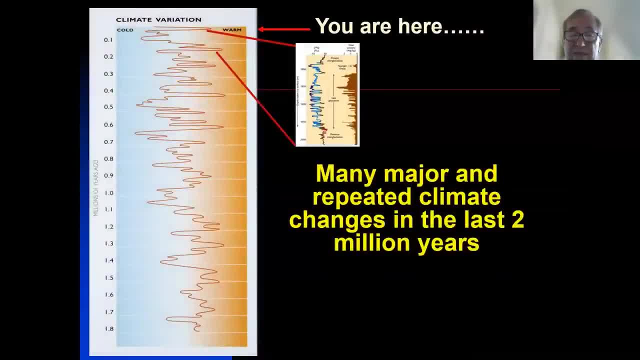 and this was a time, of course, that was affected by profound climatic changes. so here on the left we've got a an oxygen isotope curve and this shows the main major climatic fluctuations in this last two million year period. so you can see on the left there the blue colors. 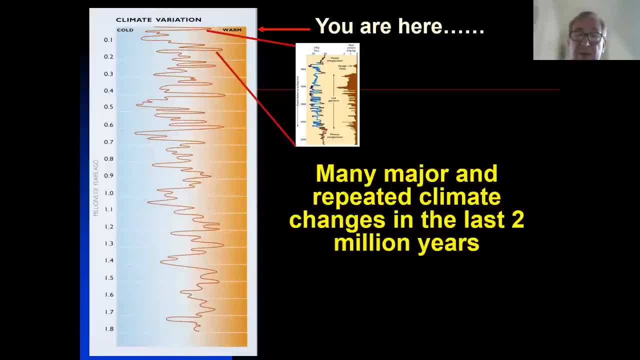 indicate times when it was cold than the present day. on the right hand side, the warmer colors show the warmer stages in this period of time and, as you can see, when we get to within the last one million years, these fluctuations become much more profound, much deeper, much more severe and it- and to really complicate matters- 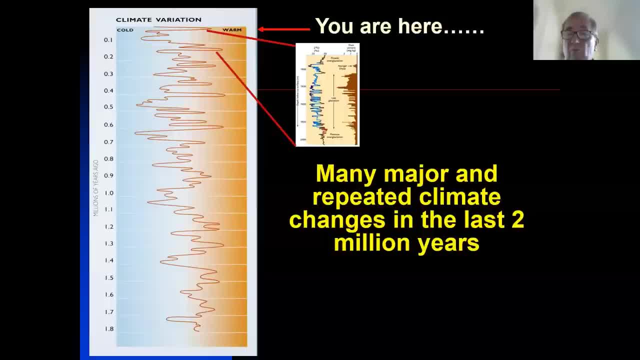 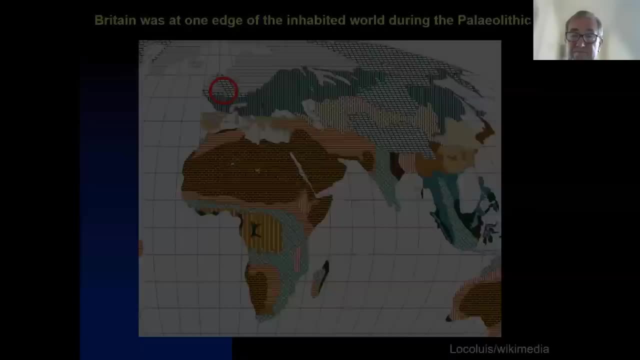 within these changes, there are even smaller, more rapid fluctuations of climate, and we can see some of those highlighted for the last 100 years. so, as humans spread out of africa, they were entering into very unstable environments, and britain, as has already been alluded to, was on the edge of the inhabited world. 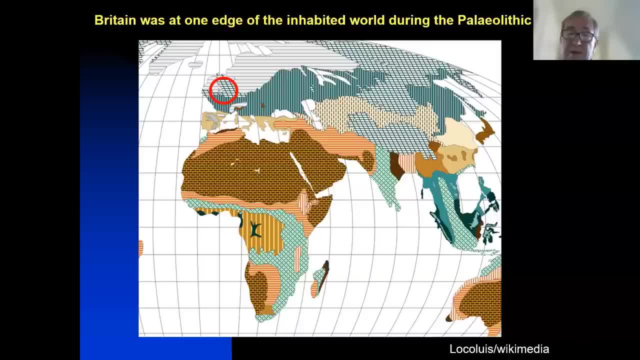 during the paleolithic. so at times we know people were not in britain at all and at other times they were here, probably in only small numbers. so britain really was on the edge of the inhabited world for most of this story, and so we can see that in the last few years 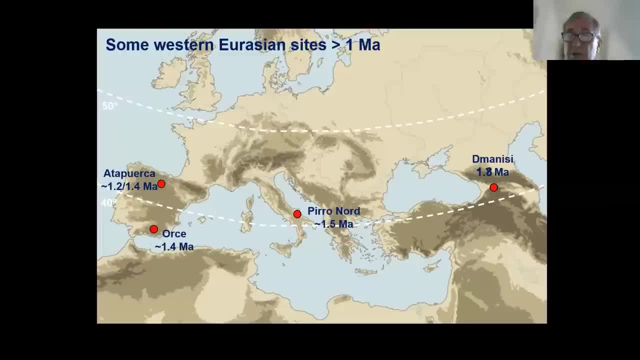 but we know humans made it into europe more than a million years ago, and so here's a mention of some of those sites. so dominica i've already mentioned, in the caucasus about 1.8 million years ago, and then in europe itself. we've got archaeological evidence from: 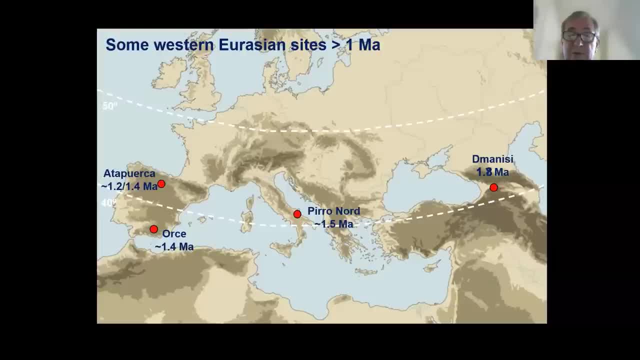 sites like piranor and we have fossil evidence from sites like orthe and atapuerca in uh in spain. but if you look at northern europe, we have nothing really showing up in northern europe for this period of time, more than a million years ago. 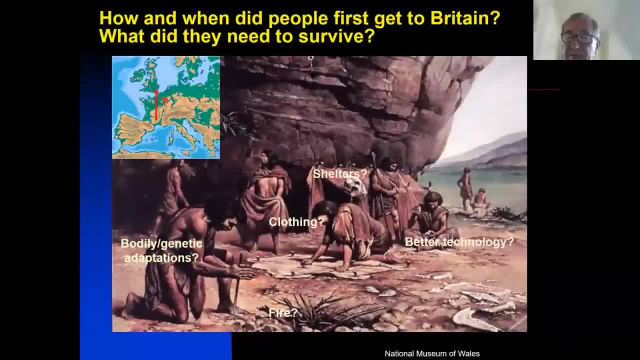 so when did people get to britain and what did they need to get there? because britain is fairly far north and it is on the edges, as we've said, of the inhabited world, so it would have been challenging for early humans. so it's assumed that to cope with the environments in places like 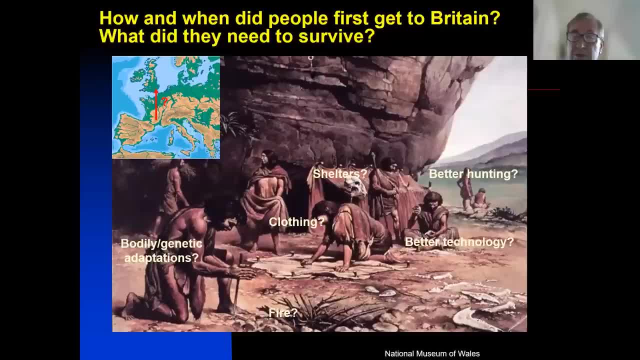 britain. humans would have needed a number of adaptations and these might have been physiological in terms of, you know, pilgrimages and people also stress to in shops, and so things like that, or even to common advice, which is just obviously more technical, but, you know, loop throughиваютour lives. 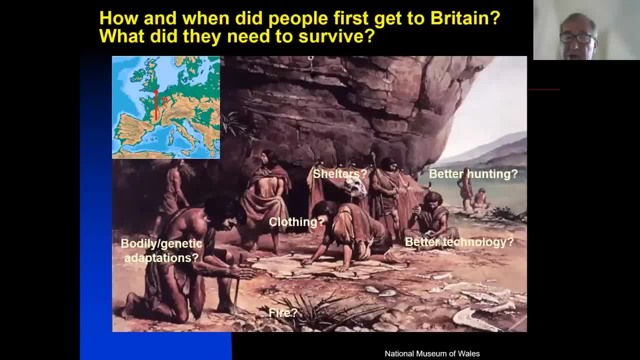 actual changes in their body physiology, in their body shape, perhaps you know, layers of fat to insulate them from the colder winters, And of course also cultural adaptations. things like clothing, shelters, better technology, better hunting, probably for food procurement possibly. 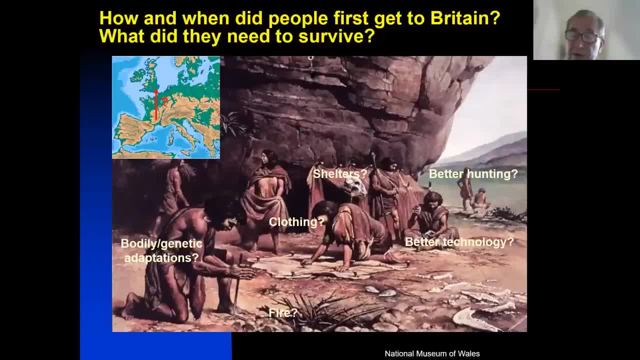 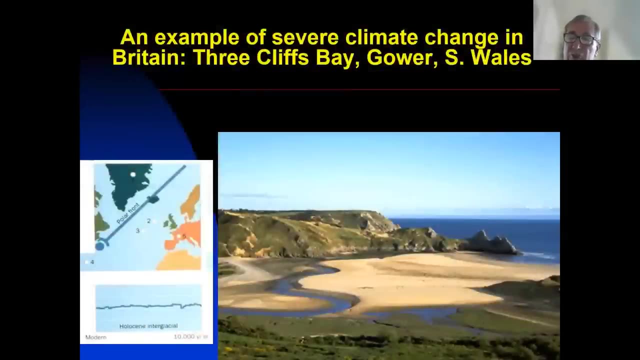 the use of fire. So these are all things that we can look for in the archaeological evidence to help us explain how humans were eventually able to adapt to these marginal and colder, much more seasonal environments. So to show how extreme things did get in Britain, I'm going to 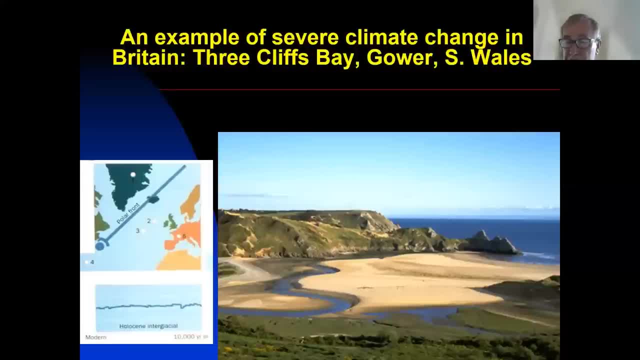 show you just an example of what's now a very nice area in southern Wales- the Gower Peninsula, Threecliffs Bay- And this is how it looks today, during our present interglacial period. So a high sea level and, of course, a mild climate. 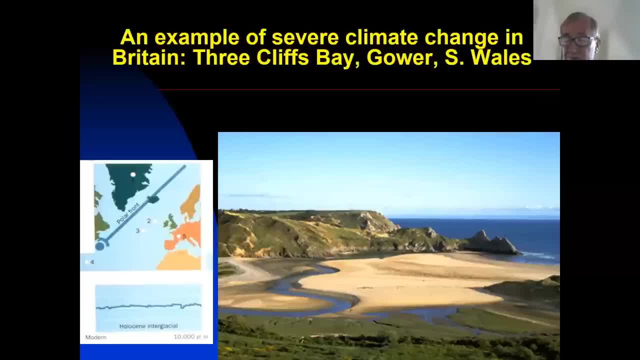 So Britain is very much influenced by the state of the Atlantic Ocean. If the Atlantic Ocean is relatively warm and the Gulf Stream is switched on, Britain has very mild winters. But when the Gulf Stream switches off, when the Atlantic is cold, things change very much. 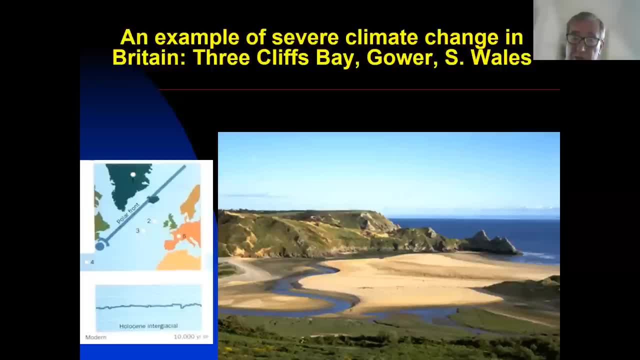 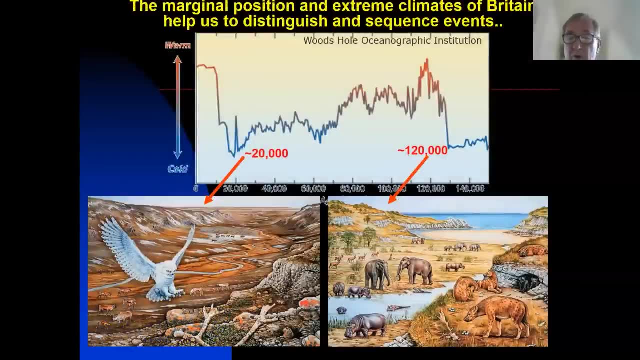 for the worse in terms of habitability for humans. So here are reconstructions for Threecliffs Bay at two times in the past. So on the bottom right there you can see a reconstruction from about 120,000 years ago, the last interglacial period in Britain, often called the Ipswichian. 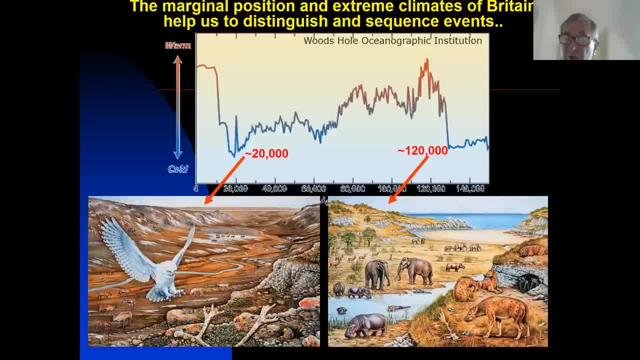 And all of the remains shown in this reconstruction on the bottom right have been found in the Gower Caves And I've been involved, and Ahob was involved, in excavating some of these sites. So we have familiar things like red deer, but we also have 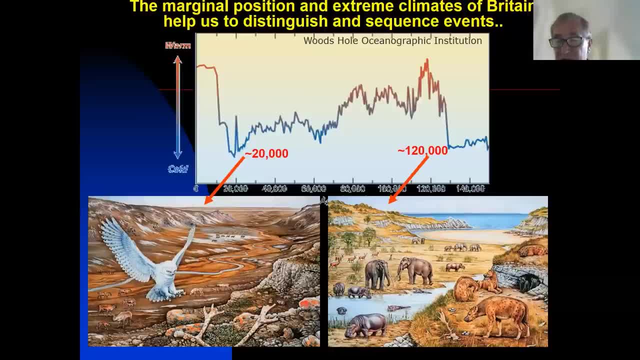 things that make it much more like an African environment. We've got elephants, we've got hippos, we've got hyenas and, you know, rhinos and a high sea level. In fact, the sea level was at times higher than it is at the present day. Summers were probably one degree warmer than they. 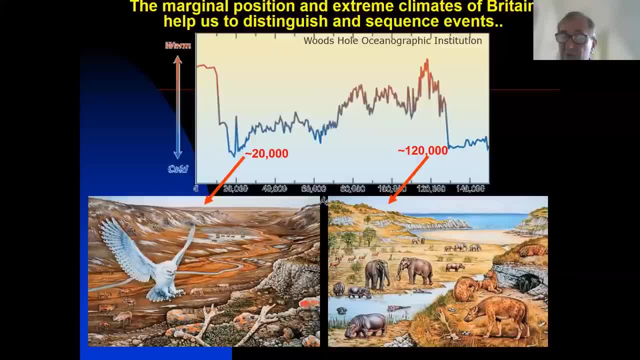 are at the present day, So that's 120,000 years ago. Let's fast forward about 100,000 years to about 20,000 years ago, the peak of the last glaciation. You can see how different the area looks now. We've got a tundra environment. 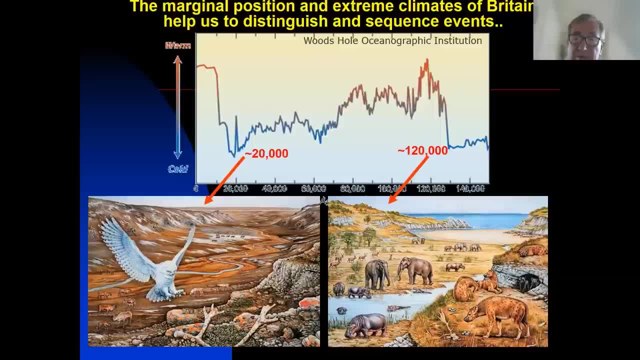 Reindeer, snowy owl, lemmings, And the sea has disappeared because the sea level has dropped. Because of the great size of the ice caps, the sea level has dropped about 125 metres, So we've got a huge coastal plain there. And one thing, of course, is very noticeable in 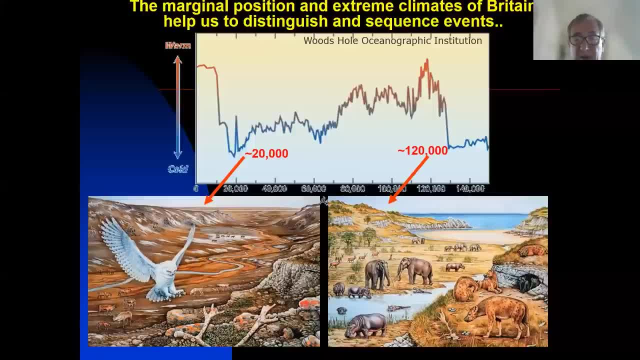 both these reconstructions. there are no people in them, And for that period, 20,000 years ago, we can guess that it just was too severe an environment for humans to survive In southern Wales at this time, And the ice sheet, in fact, was only a few miles away from. 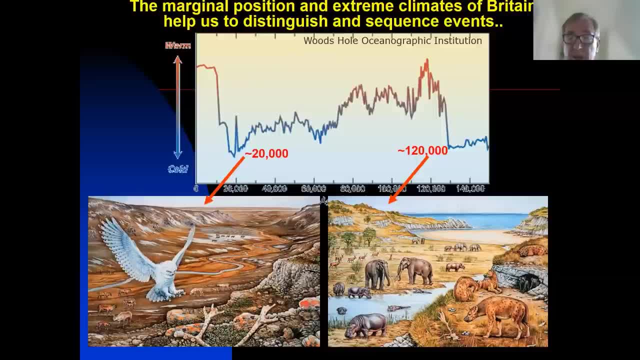 this area of Gower 20,000 years ago, But on the right hand side, the bottom right. why are there no humans there, when you would think it was a good environment for humans? Well, we'll come on to it later, But the working assumption is that Britain was an island. 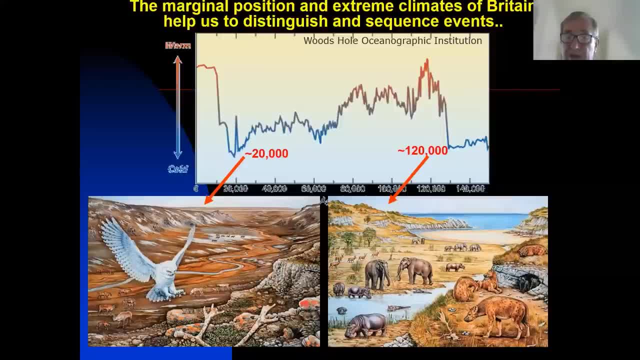 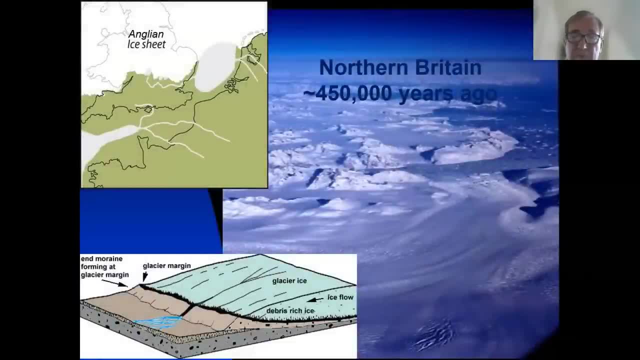 120,000 years ago. These mammals managed to get across, but humans did not. So these glaciations, when they hit Britain, were very severe, And we can see what's usually reckoned to be the most severe one, the Anglian glaciation about 450,000 years ago. So you can see the extent. 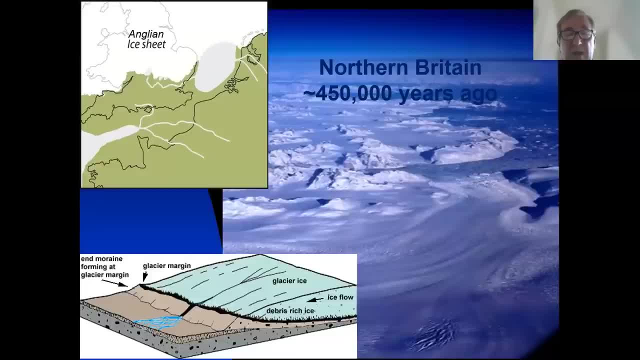 that was covered by this ice sheet. It was a massive glaciation covering most of Britain, And Britain at this time was connected to the rest of Europe by a wide land bridge, And this ice sheet, of course, moved down through Britain And it was at times two kilometres thick, massive and heavy ice sheet And it acted like. 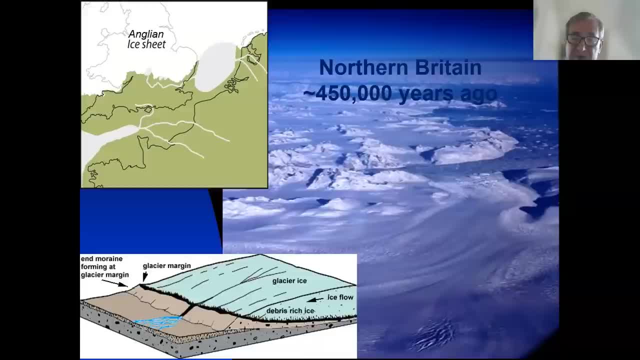 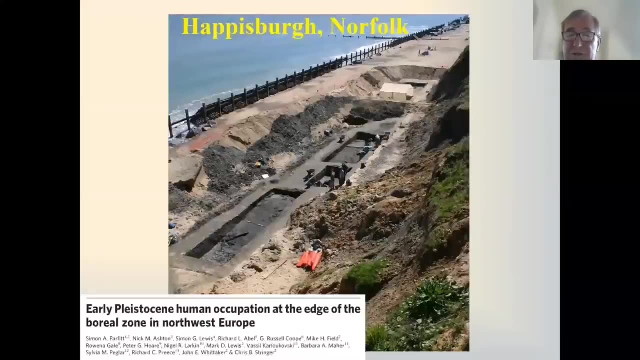 a giant bulldozer. It pushed lots of sediment in front of it and deposited that sediment at the end of its extent, as we can see in that diagram on the bottom left there, And some of that deposit of ice can be found in Norfolk at the present day. 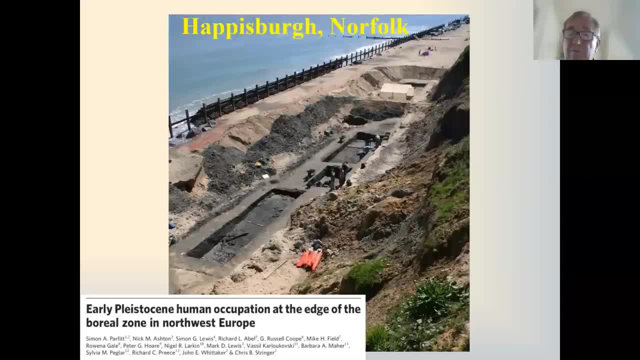 on the coast of Norfolk. So here is an illustration from Haysborough in Norfolk, And this cliff you can see just to the right-hand side is a cliff made of glacial till, So this is debris that was pushed in front of that ice sheet about 450,000 years ago. 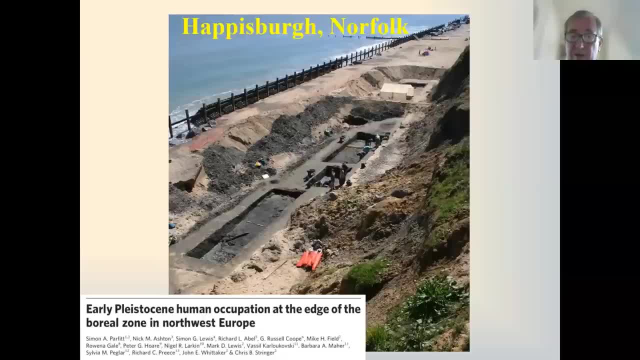 But that means that anything stratigraphically below that till must be, by definition, more than 450,000 years ago, a date for more than 450,000 years old. And you can see below the cliff. there excavations are going on, And these were led by. 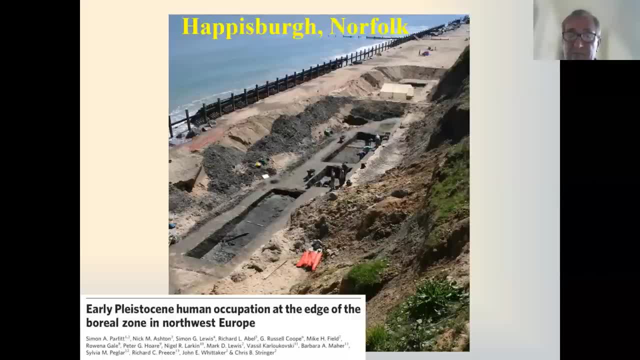 Nick Ashton and Simon Parfit and Simon Lewis, And they show a series of dark clays. And these are not sea deposits, These are not marine deposits, These are river deposits, river muds, And they've got in them large chunks of wood that's floated down the river. And so these deposits, we think 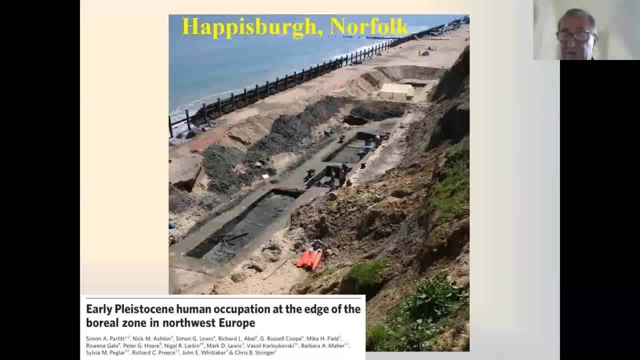 are about 900,000 years old. So there was a river flowing through here about 900,000 years ago And we think it was actually the Proto River Thames. So at this time the River Thames was flowing much further north across East Anglia and coming out into the North Sea close to this location at. 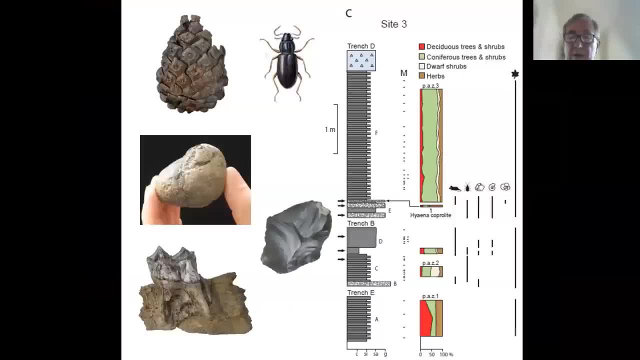 Hayesborough. So these clays are very rich in organic materials And you can see some of the material here. So this is in our paper from 2010. in Nature, There are beautifully preserved pine cones, which suggests the climate was actually more boreal. It was more. 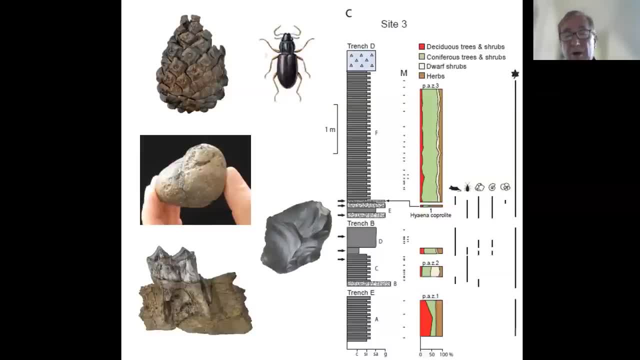 like southern Scandinavia, So perhaps more continental, with reasonably mild summers but colder winters. We have evidence like hyena coprolites, We have mammal remains And we have stone tools. So humans were there at this time in an interglacial that was probably at the downturn. 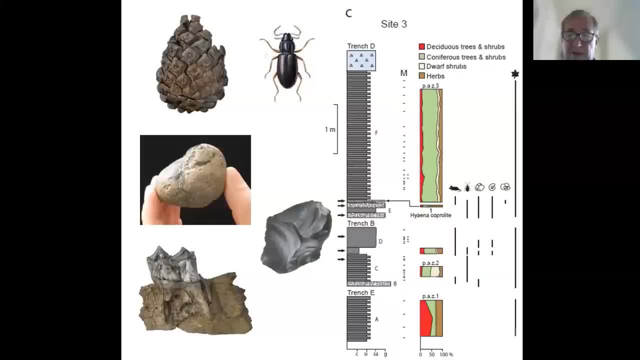 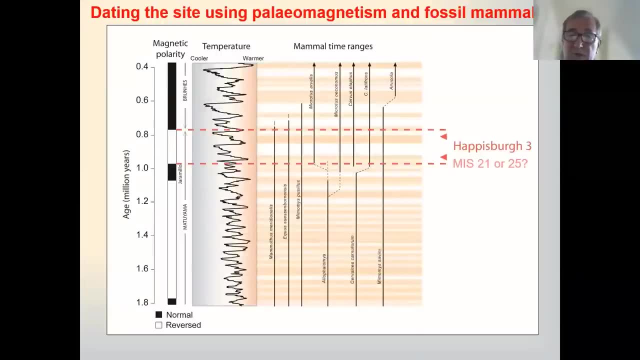 of the interglacial. It was getting colder towards the end of the interglacial. So which interglacial was it? Well, two of the main ways we're dating the site is through paleomagnetism and biostratigraphy. 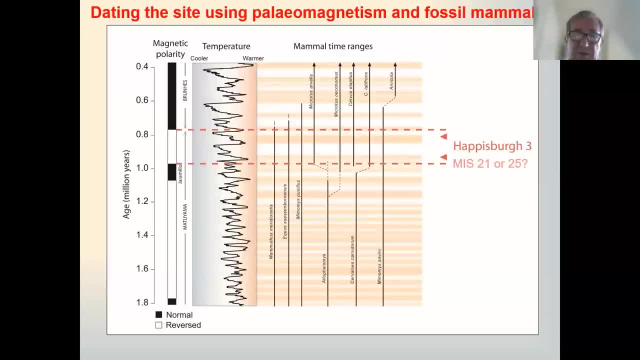 So we've got an oxygen isotope curve represented there, showing temperatures in the past, And we know that the lower parts of these Hayesborough clays are paleomagnetically reversed. The main sediments are normal polarity. So you can see here a zone between about 1,800,000 years, which is 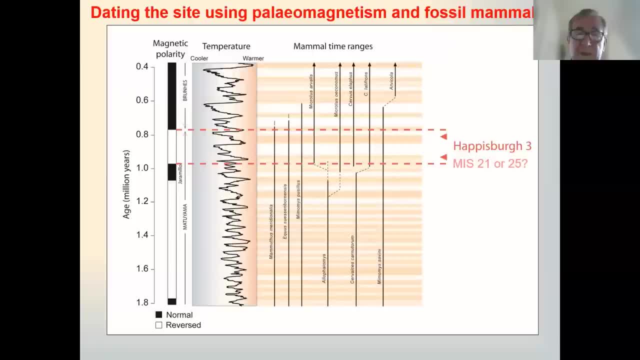 where we think the Hayesborough Three Deposits sit And through the mammal remains. we can make a shrewd guess, really, for the age of the site, because we have a number of mammals which are making their last appearances at this time in Europe And we also have another series of mammals. 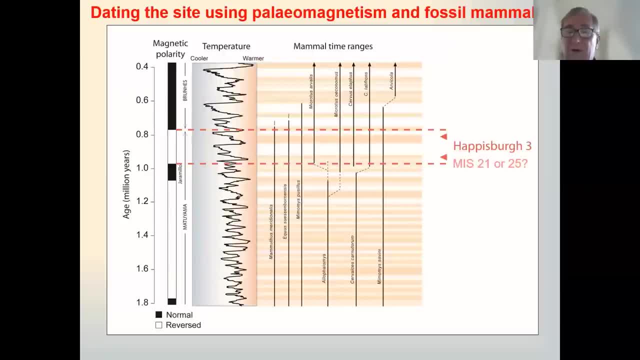 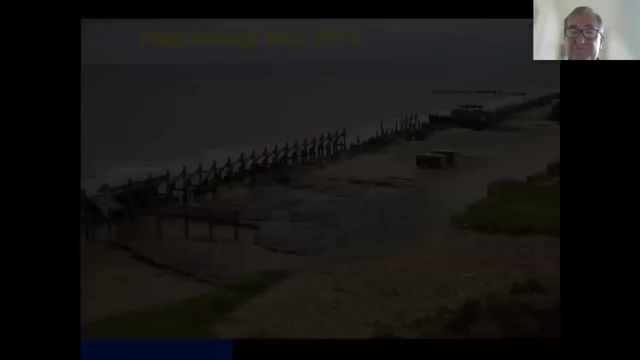 which are making their first appearances, So we have an overlap of these last appearances and first appearances, suggesting that the interglacial in question is probably marine isotopes, stage 21 or 25, around 900,000 years ago. And the Hayesborough story doesn't really stop with those artefacts from around 900,000 years. 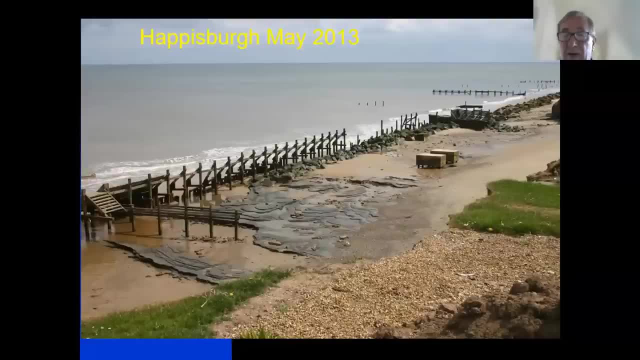 ago, which is the oldest evidence of occupation in Britain by some way. But the team were back there in 2013, taking claws to improve the dating and mapping. the sediments And those clays were outcropping and being washed over by the sea- a couple of hundred. 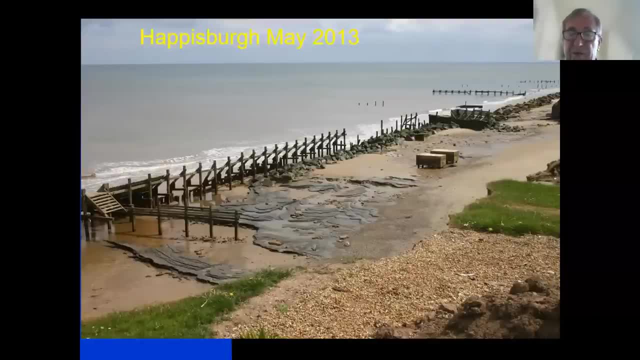 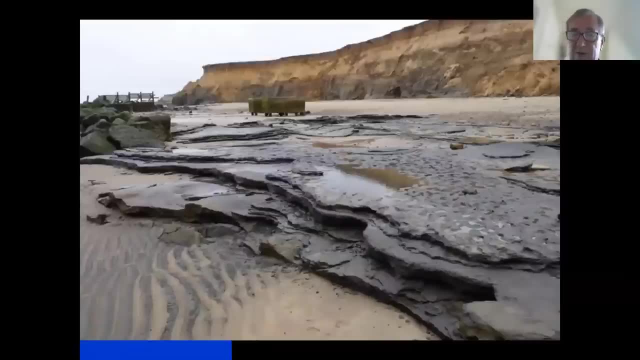 meters to the south and you can see them here on the beach, and my colleagues who were there started noticing these depressions in some of the layers of these clays- and these are really solid clays, they're not soft, so these depressions look ancient and there were a whole lot of them. 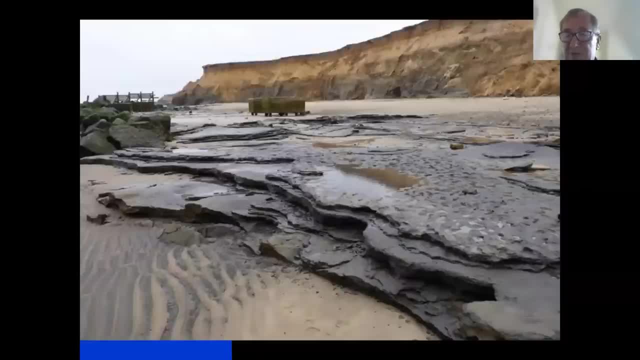 on some of the floors and they contacted us and said they thought they'd found footprints and I- I certainly was really disbelieving of this. I couldn't think the footprints could be here, and the sea was washing over them twice a day, so they'd only recently appeared. 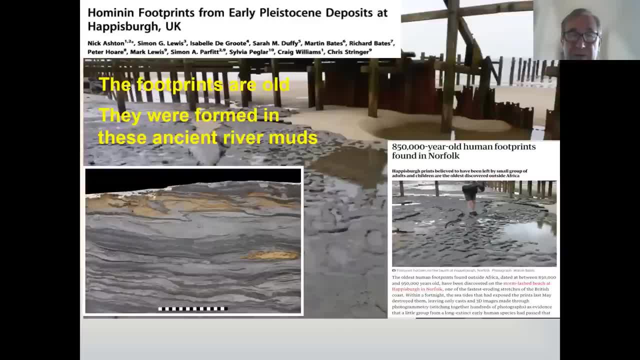 but we were able to show that these were ancient prints. they were actually embedded in the muds stratified in the clays that we could show were the same clays, by correlation, that we've been excavating at the Haysborough 3 site itself. so these were human footprints and about 900,000. 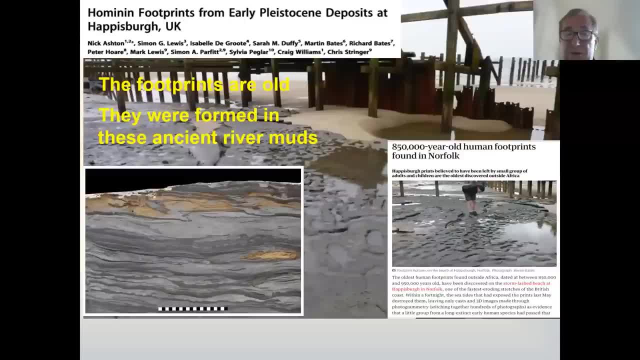 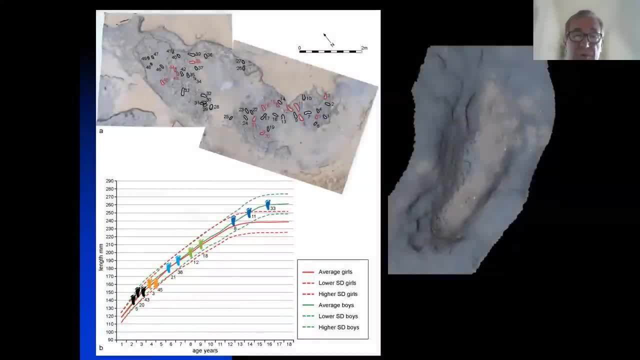 years old, so they're the oldest known human footprints at the moment, moment outside of Africa. And these prints are in different sizes. we can map them as large and small. So the suggestion is that this is a mixed group of adults and children walking. 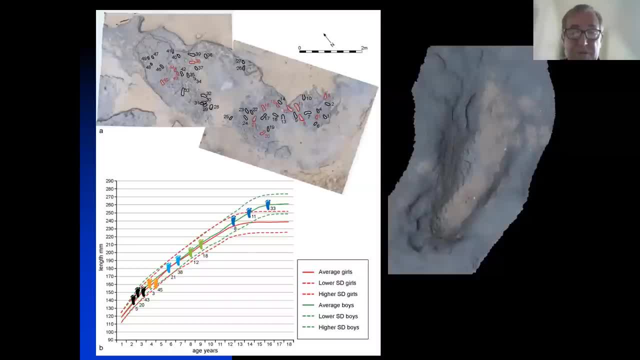 along the side of the river, probably the Proto River Thames, And you can see one of these nicely preserved footprints on the right there. If any of you are in London, we have a replica of one of these footprints in the Human Evolution Gallery. 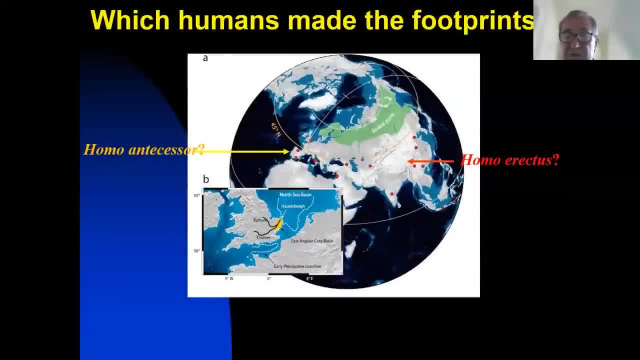 So who were these humans? Well, unfortunately we only have the footprints and the stone tools. The best guesses are, but it could be Homo erectus, which we know was around over in Eastern Asia and potentially further to the west. And, of course, 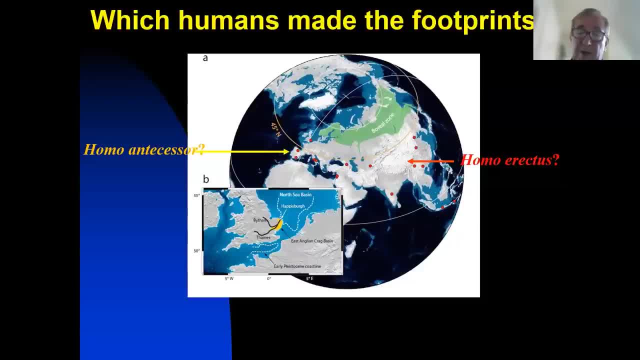 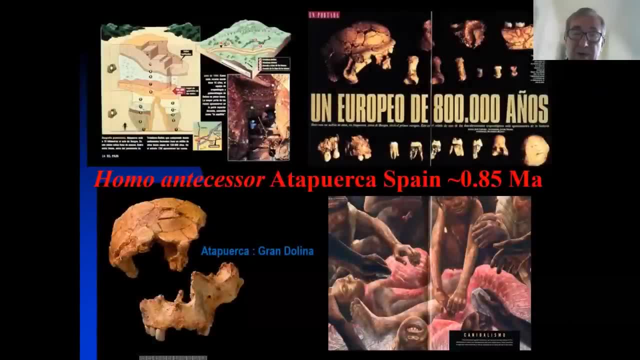 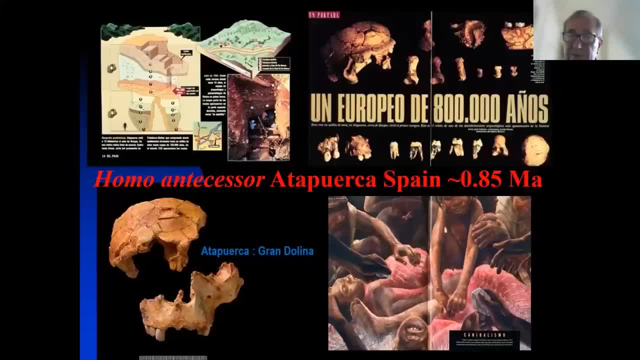 quite a substantial number of fossils, but not complete material. Much of it is immature individuals And a number of them show evidence of cut marks on them, suggesting there was cannibalism going on here about 850,000 years ago. rather gory. 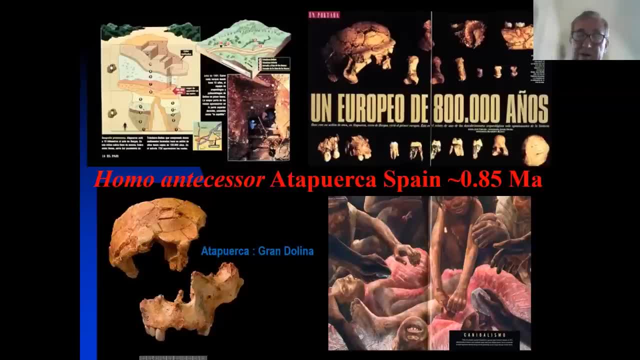 reconstruction. you can see there on the bottom right. So our best guess is that these footprints at Haysborough were being made by Homo antisessel about 900,000 years ago. But clearly it's a really. we're going to need fossil evidence to really 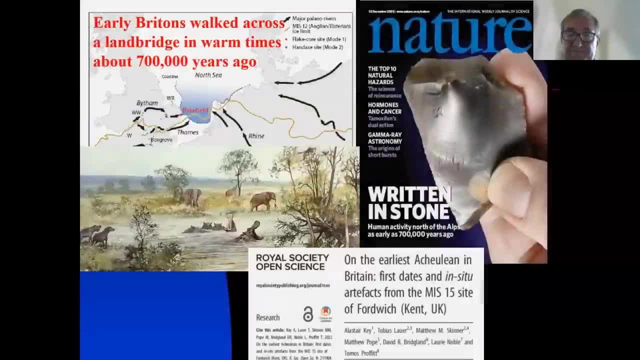 demonstrate which species was there. And then, moving on in time, we have an occupation represented by archaeology about 700,000 years ago. And at Pakefield in Suffolk, again, coastal deposits. we were able to recover artifacts and cut mark bones from the site of Pakefield. And here the climate. 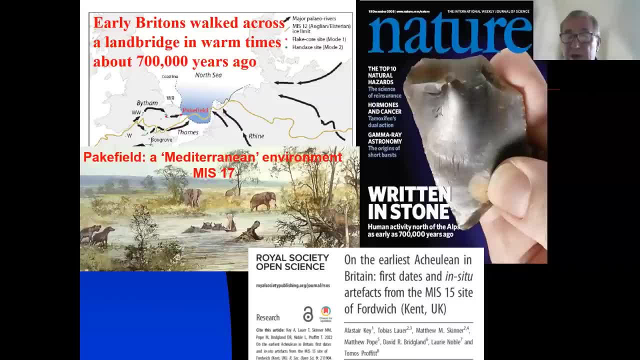 was a warmer climate. it was much more Mediterranean. we can tell from the fauna and the flora That this was a site that had a Mediterranean like environment, with warm summers and cooler, damper winters. so dry summers, dry warm summers, cooler, damper winters, and humans were 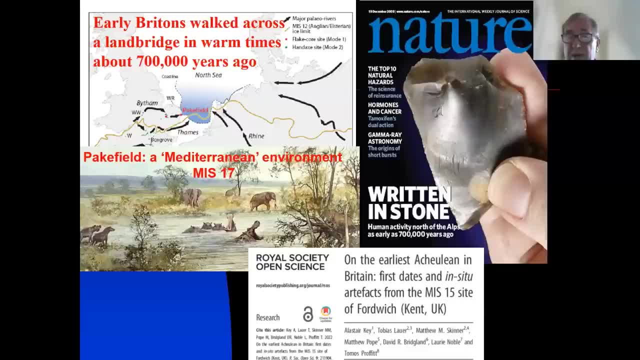 there at this stage making flake tools. And then, when we come on to around 600,000 years ago, MIS-15 recently published evidence suggests that humans were indeed there as well, And we actually have some of the earliest hand axes in Britain. 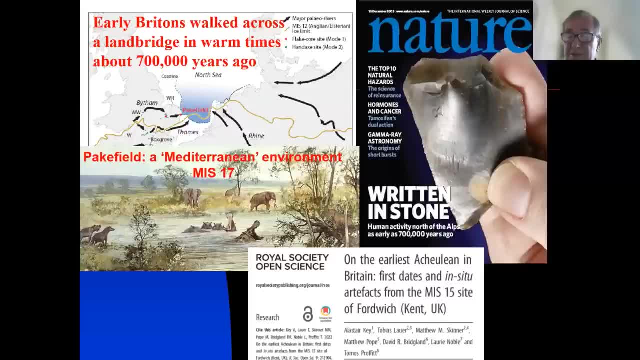 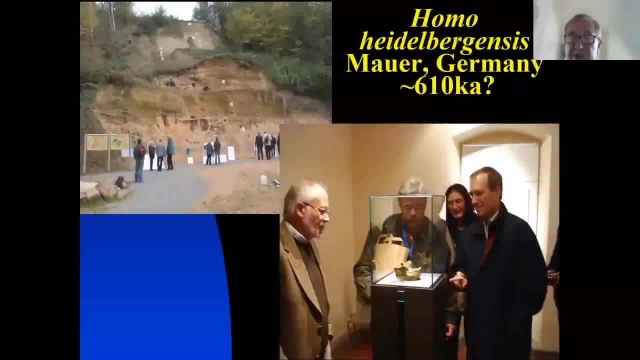 known from the site of Fordwich in Cairns, Kent, from about 600,000 years ago, And because that date correlates well with the date in Germany of the Mauer Mandible, so here we are worshipping the mandible at its 100th anniversary earlier, earlier in this century in. 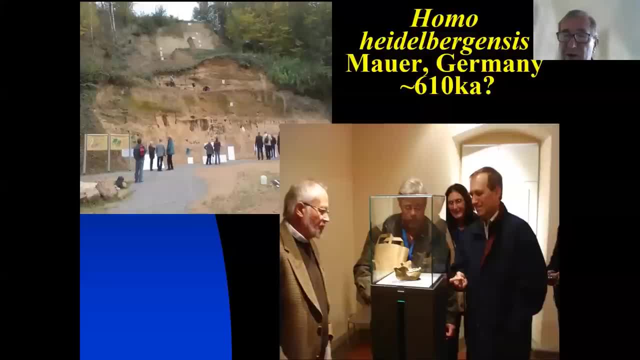 Germany. the Mauer Mandible found in the Mauer sandpit near Heidelberg and of course, given the species name Homo heidelbergensis in 1908. Dated radiometrically to about 610,000 years ago. So possibly this was the. 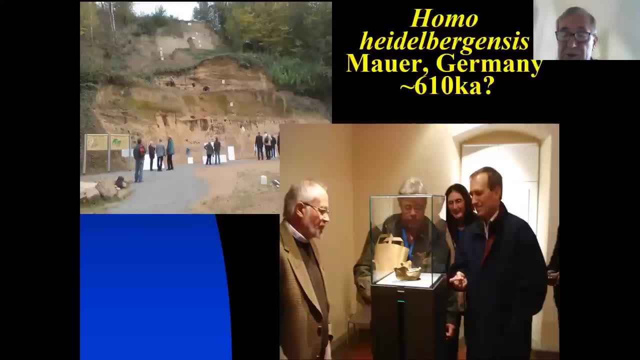 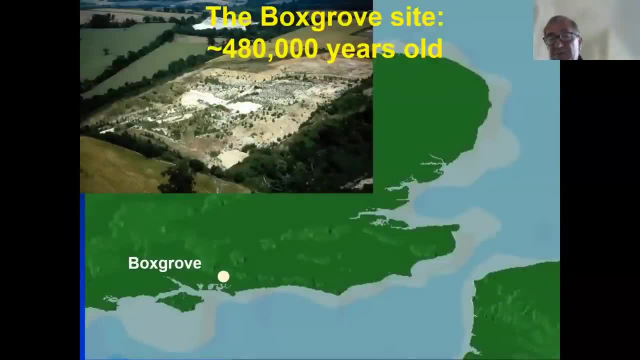 species that was in Britain making those hand axes at Fordwich, but we can't be sure. And now, moving on to the next interglacial, So this is MIS-13. now We have humans present at Boxgrove and this is a wonderful site. that was. 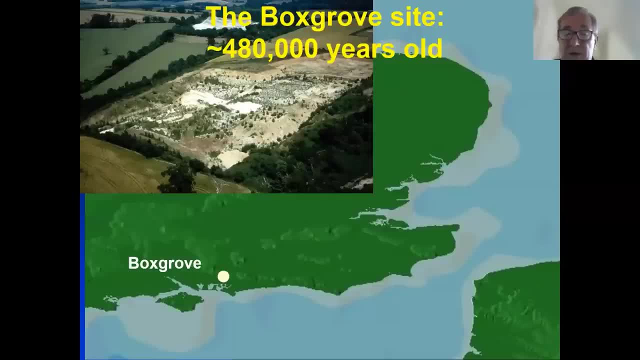 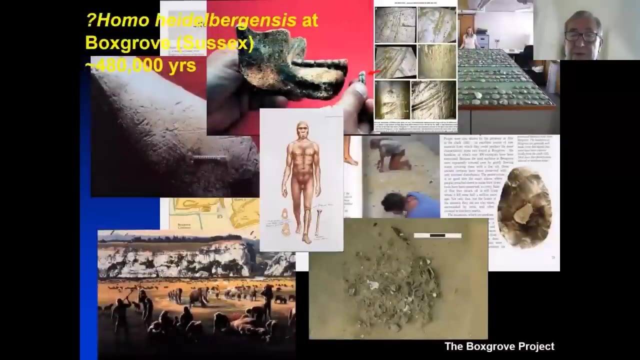 excavated mainly in the 1990s close to the south coast near Chichester. At this time the sea was further north and was cutting into the chalk cliffs there and humans were there and a very rich fauna. So here's some of the evidence from Boxgrove, courtesy of the Boxgrove project, and 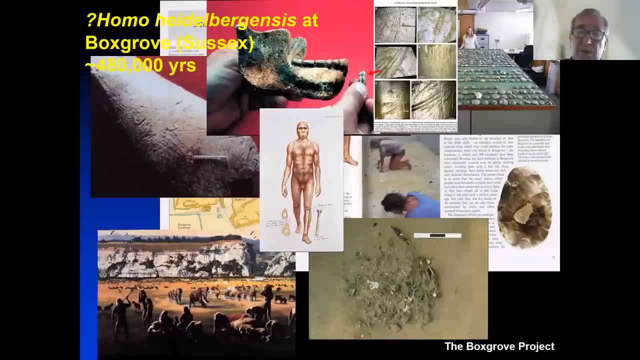 some of the members of the Boxgrove project were members of AHOB, So we have beautiful scatters of flint debris showing where people were napping hand axes using the chalk, from those using the flint, from those chalk cliffs. About 400 hand axes have been recovered there. You can see some of them. 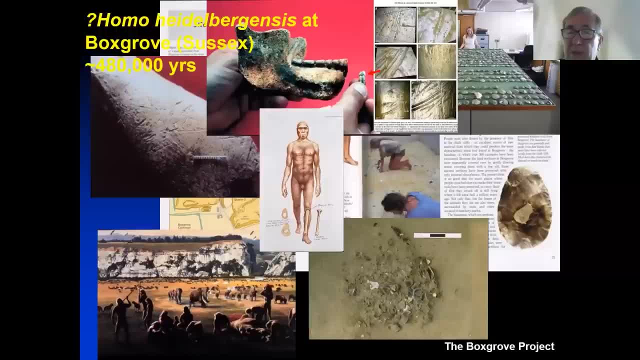 laid out on a table at the British Museum. We've got cut mark bones of animals like deer and horse. even rhinoceroses were being butchered at Boxgrove about 480,000 years ago and we're lucky enough to have some fragmentary human fossils. There's a shin bone, a tibia, a left tibia. It's lacking. 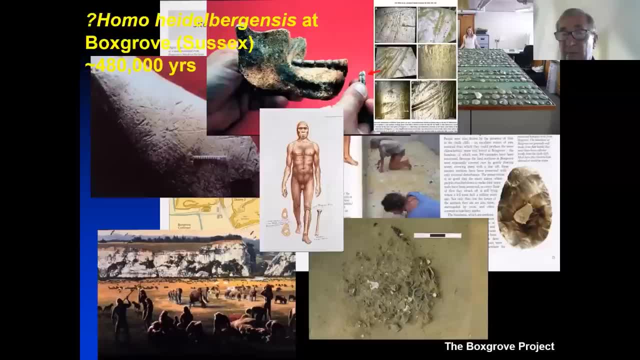 its ends very strongly built, very robustly built, And a couple of incisor teeth which look, as you can see, quite similar to the ones in the Mauer mandible. We've got a replica of the Mauer mandible there, compared with one of the incisors. 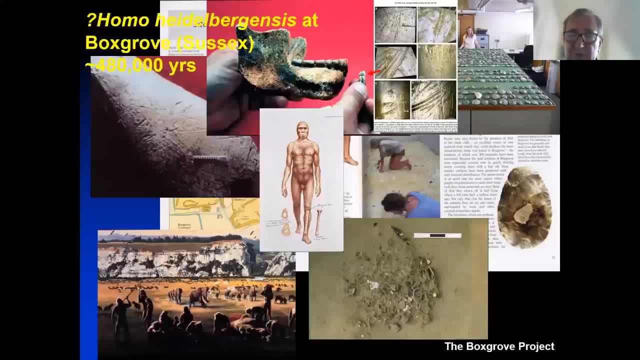 from Boxgrove, So we published this material as probably representing Homo heidebergensis, but of course we don't have a mandible from Boxgrove to compare with Mauer, so this was really a guess based on a dating correlation and we obviously need better evidence of who's there and 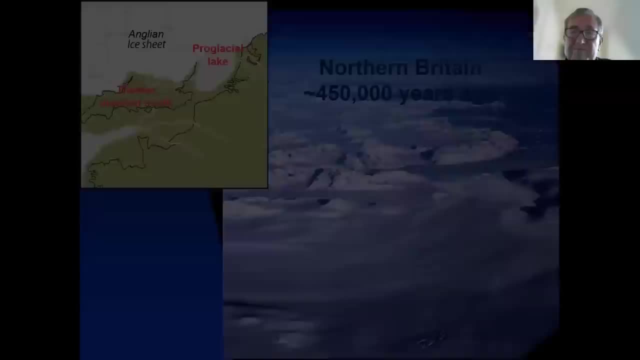 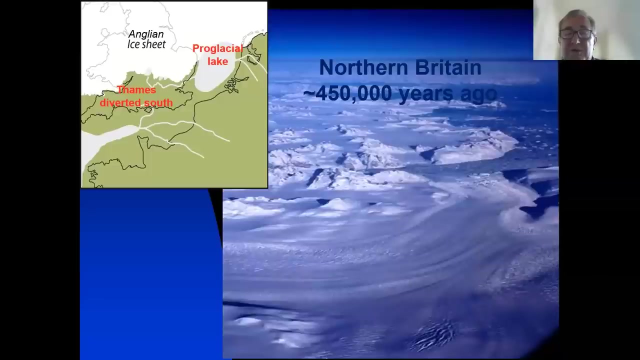 I'll come back to that question. So we now have that major glaciation following on from Boxgrove, So the Anglian ice sheet covers much of Britain. The River Thames is diverted southwards towards its present course and we get the build-up of a huge lake where the North Sea is today. And that lake was being fed both by: 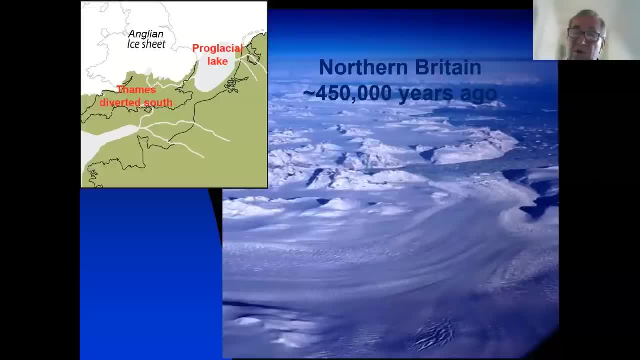 melt waters from the glaciers and also by rivers flowing into that lake. So this lake increased in size. until at some point in the 19th century, when the Great Barrier Reef was built, it was the largest lake in the world And at that stage, around 450,000 years ago, there was a massive 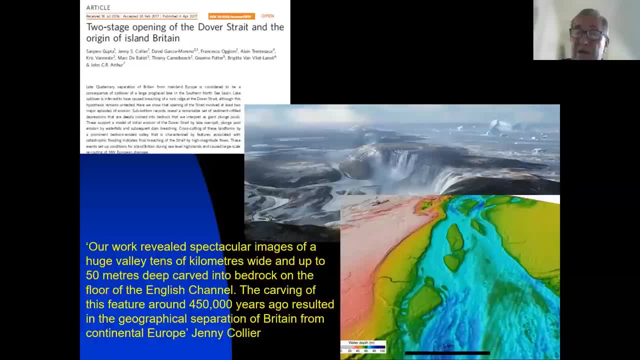 catastrophic flood which represents the beginning of the formation of the English Channel as we know it today. So this was a work led by Sanjeev Gupta, and you can see a quote here from one of the co-authors, Jenny Collier. Our work revealed spectacular images of a huge valley, tens of 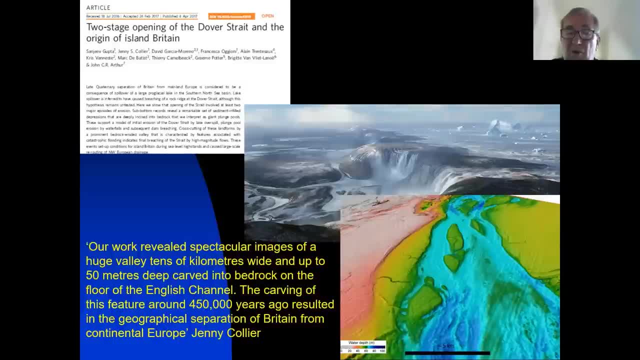 kilometres wide and up to 50 metres deep, carved into bedrock on the floor of the English Channel. The carving of this feature around 450,000 years ago resulted in the geographical separation of Britain from continental Europe, So this was a massive, catastrophic event. We think that the 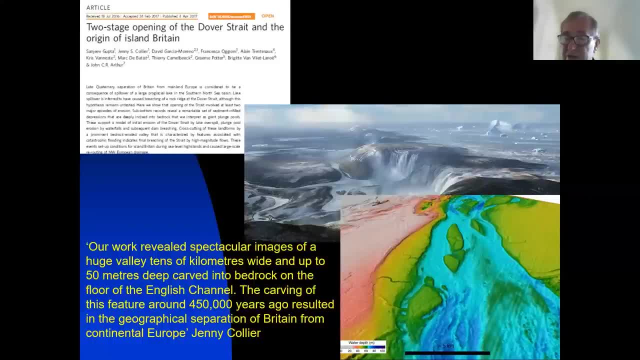 actual channel as it is now was cut in several stages, So it did not immediately form the shape and depth it has today. But this was the beginning of the formation of the channel And it meant that whenever you had a very high sea level, there was the potential that Britain could be isolated from. 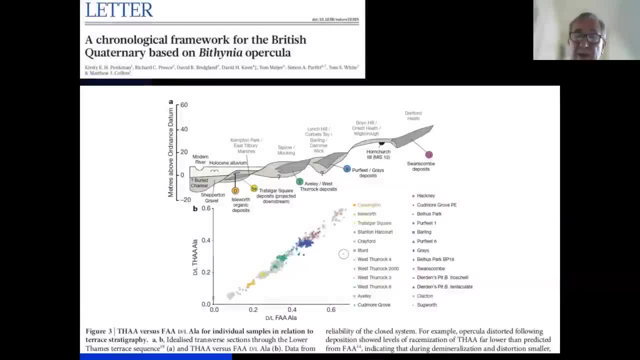 the rest of Europe. And when we move on in time now to MIS 11,, about 400,000 years ago, we have what has been described by David Bridgeton as a staircase of terraces alongside the present course of the River Thames. And you can see this staircase of terraces And as you walk up that staircase of 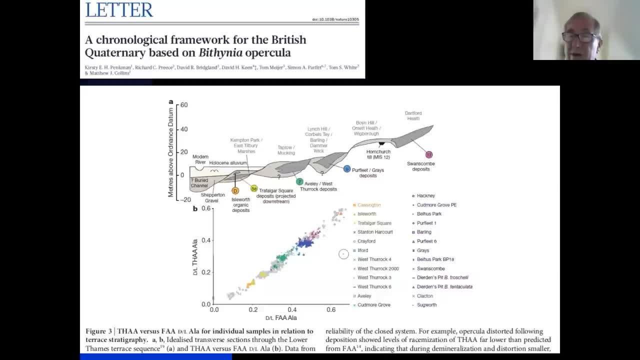 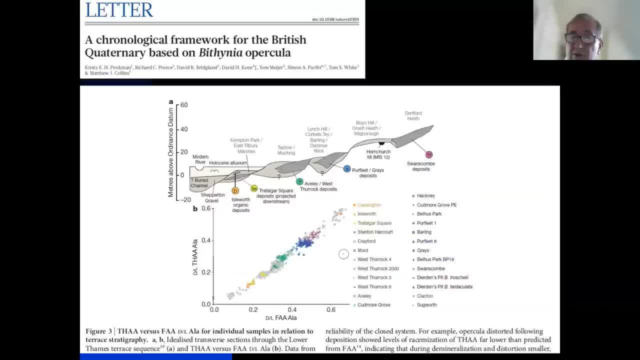 Deposits, I hope, representing the river Thames, And at the top of those you can see the Swanscombe, Averly and at Trafalgar Square. So Thirsty Penkman and colleagues have done some wonderful work looking at amino acid ratios of Bithynia opercula. So these little bits of mollusks can be used. 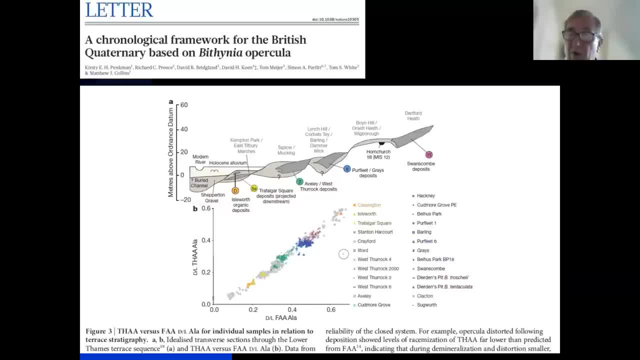 to get amino acid data which allows you to develop a clock to date these sites, And this very nice paper published about 10 years ago in Nature shows how you can use the amino acid data to really date these terraces really quite precisely in their order. 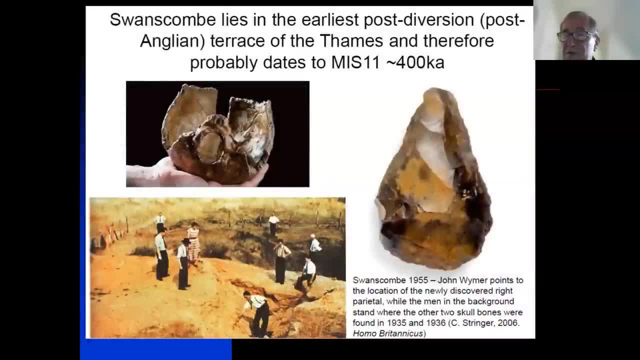 And so we think that Swanscombe dates from the first terrace laid down after the Thames was diverted close to its present course, So after that major cold stage about 450,000 years ago. So the Swanscombe site, the Swanscombe human, and here we've got these three bones of the Swanscombe. 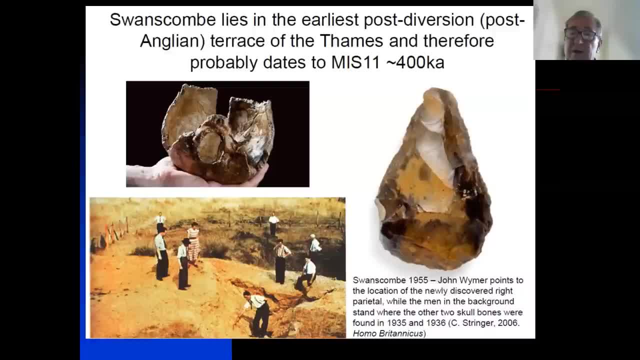 skull, the back of a skull found starting in 1935, remarkably found in three pieces at three different dates and they fit together perfectly to form the back of a skull. It's quite likely that the whole skull was there and, sadly, was not. 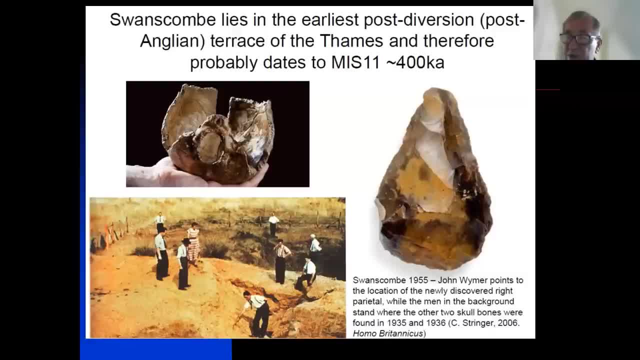 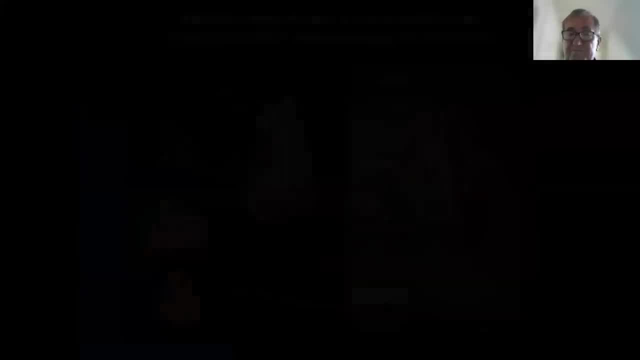 not recovered. We only have these three bones and associated with it in the middle gravels at Swanscombe, tens of thousands of these beautiful hand axe tools. And what's interesting is that at Swanscombe you have an archaeological succession. so the middle gravels. 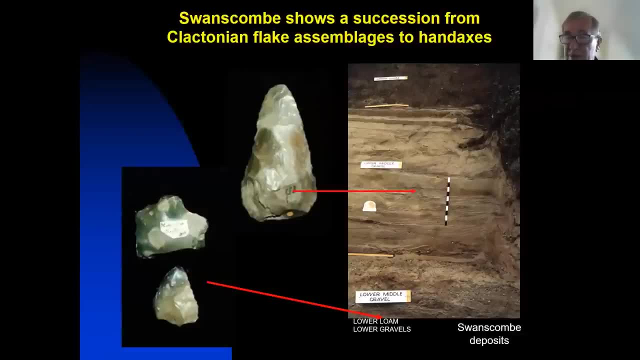 with the Swanscombe skull and the hand axe. tools can be mapped as you can see there in this diagram. but below them, in the lower loam and the lower gravels, you don't find hand axes, but you find clactonian artifacts, and so there's this interesting archaeological succession. 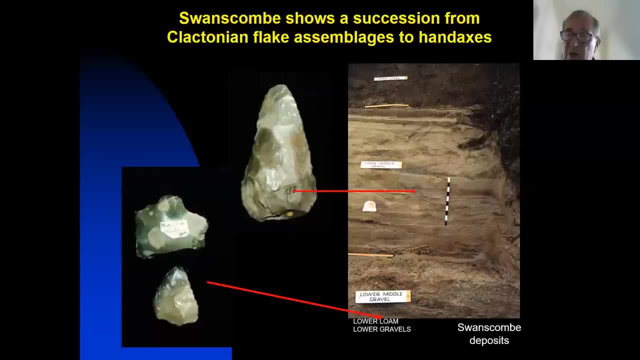 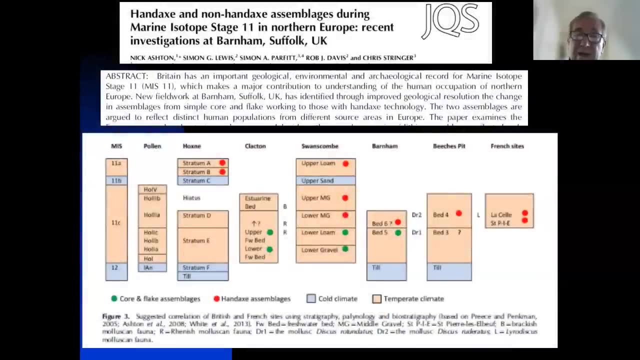 industries without hand axes, succeeded by industries with hand axes and then with the Swanscombe human and Nick Ashton and colleagues have done some very nice work mapping this kind of pattern across Britain in general, and so there are a number of sites where it seems there is a. 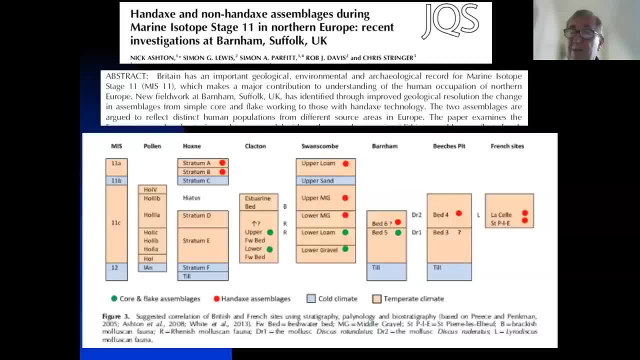 succession of clactonian artifacts in MIS-11, succeeded by Acheulean, by hand axe tools, and of course we wonder whether there might be two populations involved. as it says here, new fieldwork Barnum has identified, through improved geological resolution, the change in assemblages from simple 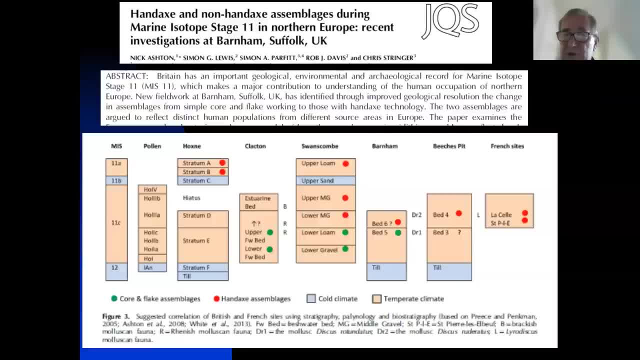 core and flake working to those with hand axe technology. the two assemblages are argued to reflect distinct human populations from different source areas in Europe. so we would argue on the strength of the Swanscombe human that there was an early Neanderthal like population associated with. 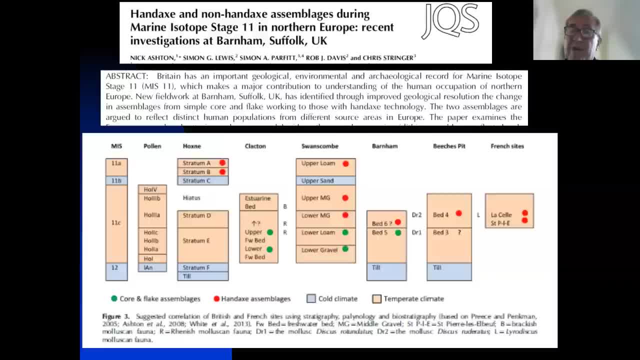 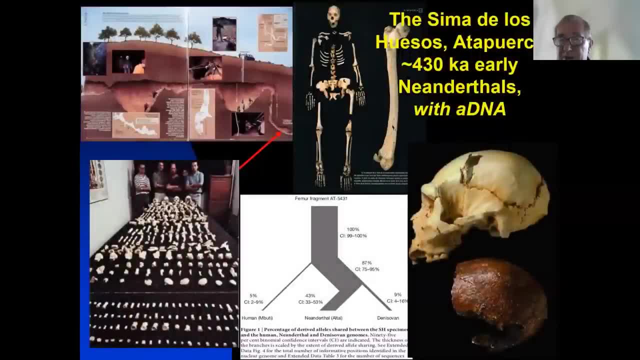 the hand axes. we don't know who was making the clactonian artifacts, and that's one human on the bottom right there, a replica- compared with one of the wonderfully preserved skulls from Atapuerca, from the Cima del Huesos. so of course this is an assemblage found. 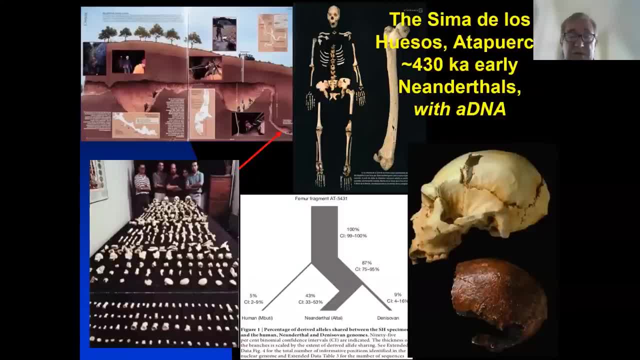 deep in the cave system at Atapuerca. over 6 000 human fossils have been found there, representing, I think at the last count, 28 or 29 individuals. every bone of the skeleton is represented and the skulls seem to match the ones from Swanscombe. really quite well, they show some Neanderthal like. 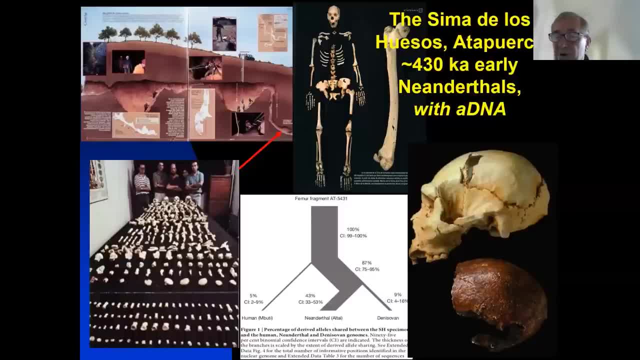 features in having, for example, a super-iniac fossa on the back of the skull, and even DNA, of course, from a couple of fragments from the Cima de los Huesos shows that this material appears to be on the Neanderthal lineage, although, as we heard in the talk just before mine, of course- 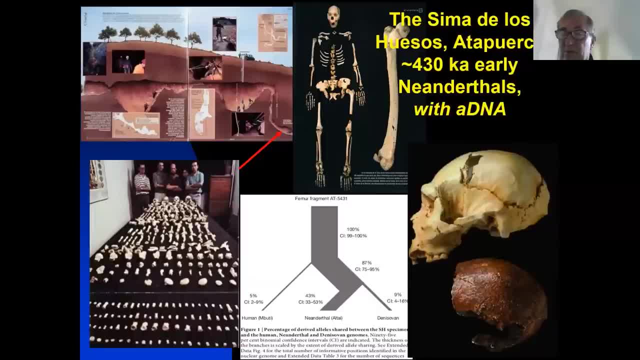 in the ear bones. there's evidence that, yes, these are Neanderthal like but also have an have some actual distinct features suggesting they might not fit neatly as direct ancestors for later Neanderthals, but certainly part of the Neanderthal clade, along with the Swanscombe. 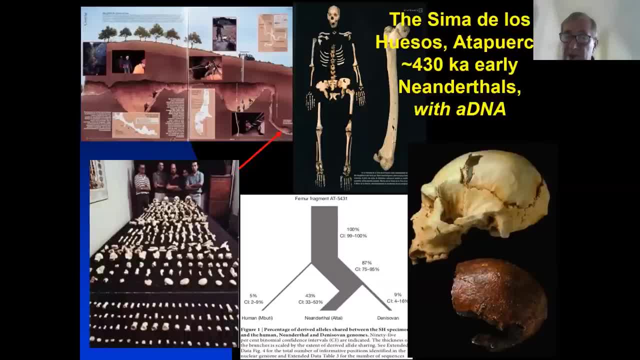 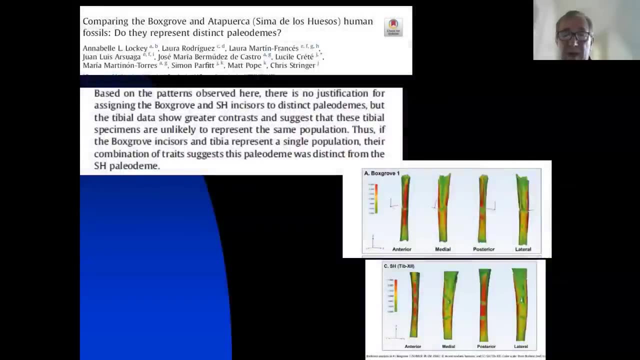 human who seems to represent a very similar population. So these are people then in Europe around 400 to 430,000 years ago and apparently early members of the Neanderthal clade. So we use this sema material to look back at the Boxgrove material because, of course, 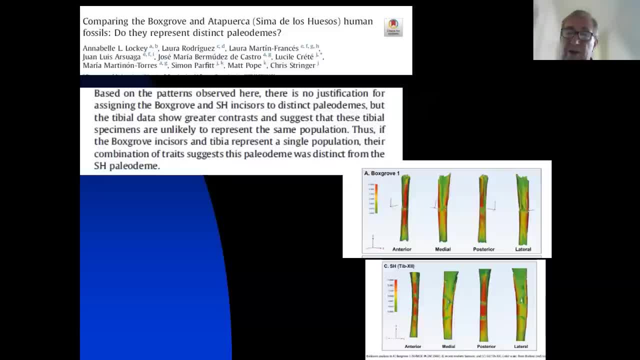 you've got a nice sample of tibiae from Atapuerca and you've got a nice sample of incisor teeth from Atapuerca. So we recently did a comparison with our colleagues on the Atapuerca team of the Boxgrove fossils. 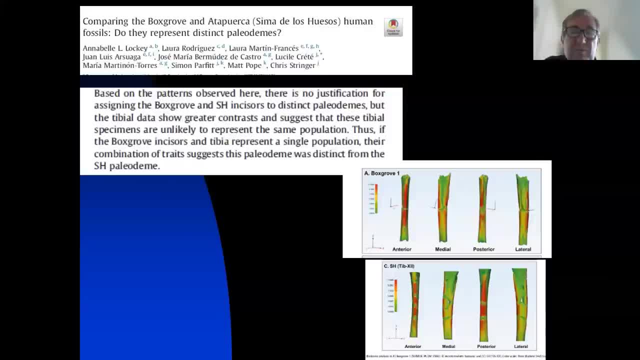 and what we were able to say then is that, as it says here in our paper from JHE, there's no justification for assigning the Boxgrove and sema incisors to distinct Palaeodebes, distinct populations. But the tibial data show greater contrasts and suggest that these tibial specimens are 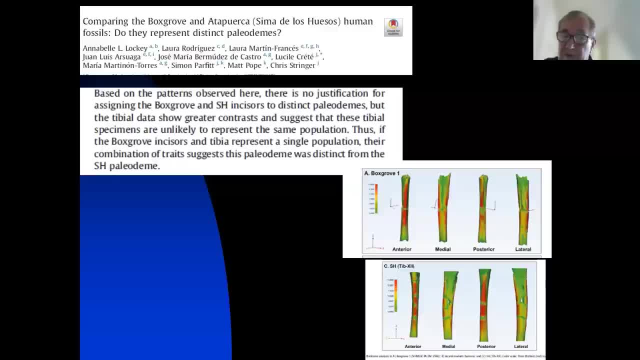 unlikely to represent the same population. Thus, if- and it is a big if- if the Boxgrove incisors and tibiae represent a single population and they were found at slightly different levels at Boxgrove, if they represent the 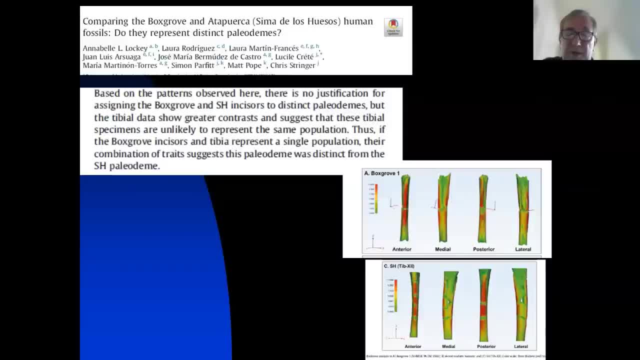 single population. their combination of traits suggests this Palaeodebem was distinct from the sema Palaeodebem. So the sema Palaeodebem in the tibiae certainly shows some Neanderthal activity. However, if we look at the Neanderthal features, those are less obvious in the Boxgrove tibiae. 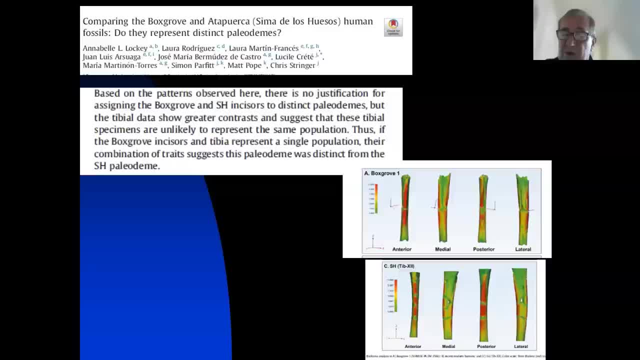 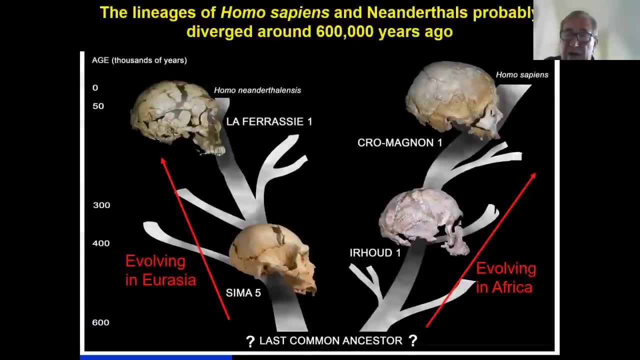 So maybe there is evidence here of some population separation between Boxgrove and the sema people. So of course, looking at the bigger picture, we think that the Homo sapiens clade was evolving in Africa over the last few hundred thousand years ago, while the Neanderthal clade was. 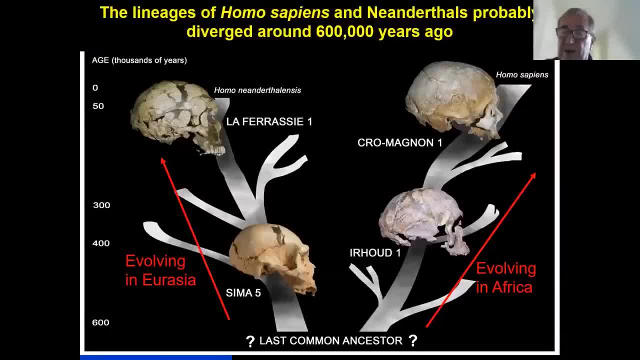 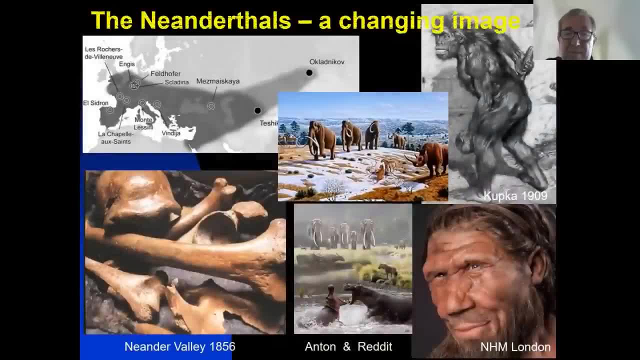 evolving in Eurasia and as we look at the European record and the British record, we can see this evolution of the Neanderthals through time. So of course the Neanderthals are very well known humans and I can't spend much more time. on them, But of course we know they covered a wide range beyond Europe. it's probably wrong to see them as as especially European humans. their range extended across into Western Asia and, we know, at times into Siberia. I think it's possible they even got into places like 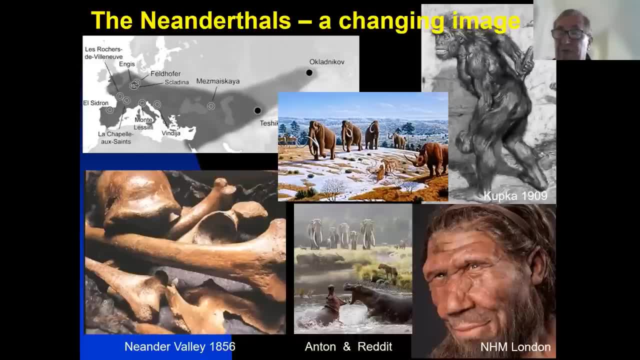 China at times We don't really know. They were highly evolved humans and they were not just cold adapted humans. they certainly were alongside the kind of fauna we can see in the beginning, in the middle of this diagram here, But also we find them at times with the fauna in the centre of the diagram, at the bottom. 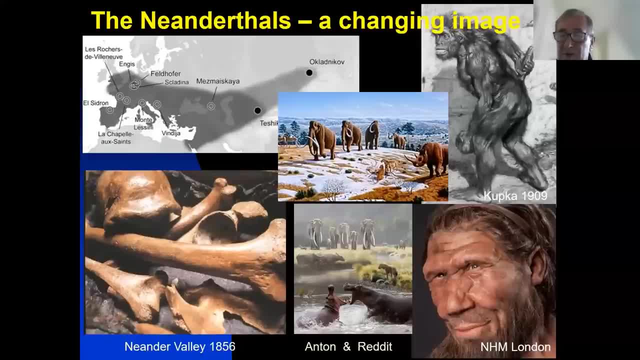 there. things like Straitus, elephants and hippos and Neanderthals were certainly not just cold adapted. they lived during the warm winter glaciers and there's some evidence that actually they did very well During the interglacials in Europe. 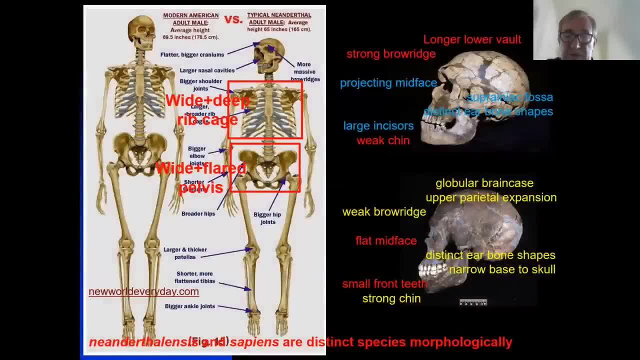 But of course they're distinctive humans, in my view, a distinct species of human from us, And we can see here Neanderthal skeleton compared with the Homo sapiens skeleton, a composite, and on the right there we can see at the top a late Neanderthal cranium compared with 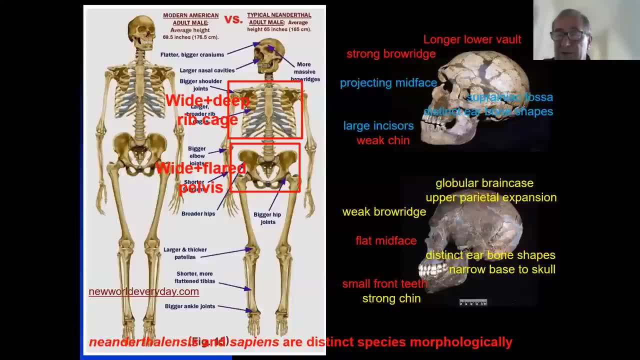 an early Homo sapiens cranium And so we can see characterised there in those crania on the right hand side In red In red we've got primitive features that these crania show, for example the longer lower vault of the Neanderthal brain case, the flat midface of the Homo sapiens. we think 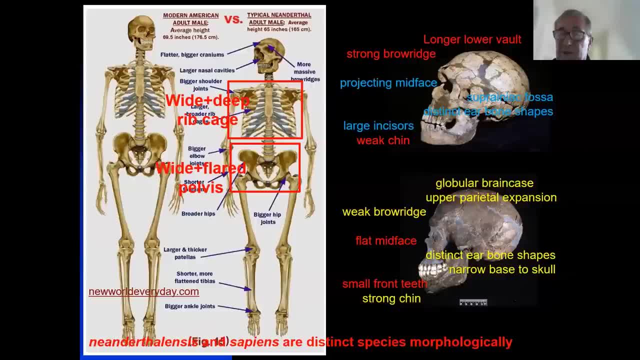 are primitive features And then there are distinctive derived features. So in blue there we've got the Neanderthal derived features, such as the projecting midface, the distinct ear bone shapes that we heard about a bit earlier, And for Homo sapiens, of course, we've got this globular brain case inside view and 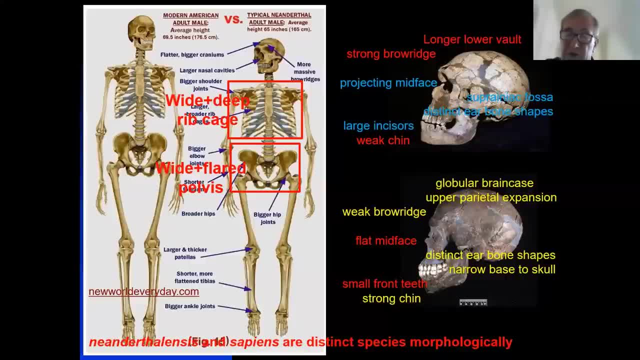 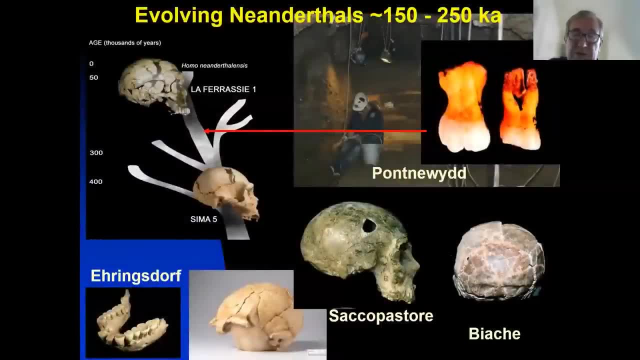 the weak or non-existent brain case, And then we've got a strong chin on the lower jaw. So I think there's enough to make Neanderthals and Homo sapiens distinct species. but we'll come back to that question if there's time, a little bit later. 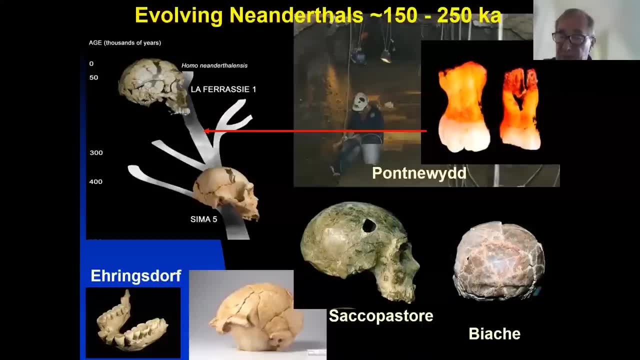 So through time we can map the evolution of the Neanderthals in Europe and now and again even in Britain. So we have early Neanderthals such as those from Sacro Pastore, probably from MIS 7, from Eringsdorf. 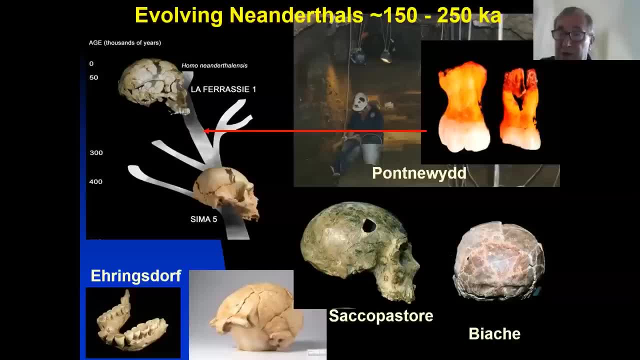 We have from Biache in France, perhaps MIS 6.. In Britain we have a number of teeth from Pont Neuwirth, over 200,000 years old, And these show a lot of Neanderthal features, as well as closely resembling the teeth from. 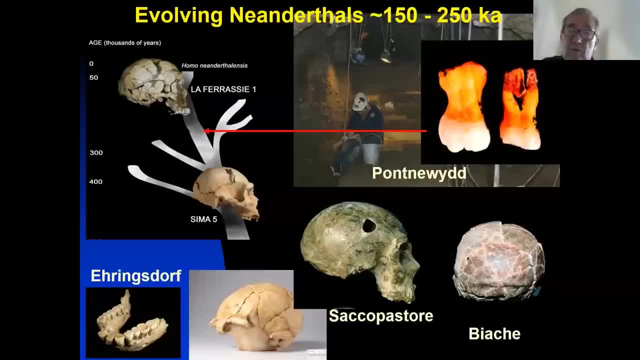 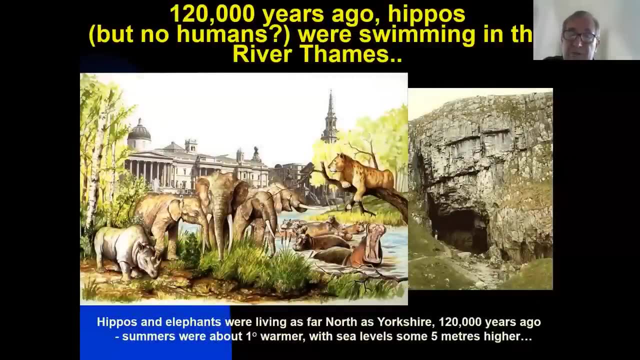 the Cima de los Huesos. So when we pick up fossils now, we're picking up Neanderthal-like fossils in the fossil record of Europe, And then we come to this interesting period about 120,000 years ago When it seems there was a rich fauna in Britain, an interglacial fauna with hippos. 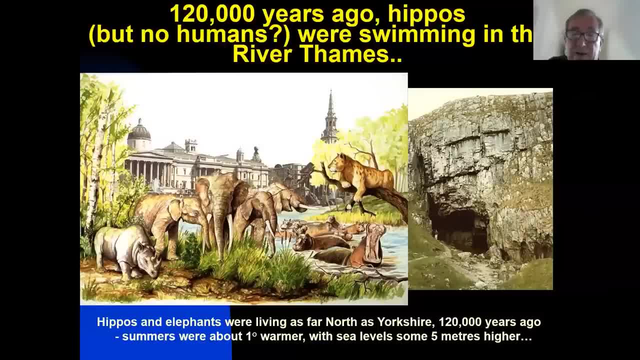 and elephants. And here's what Trafalgar Square might have looked like 120,000 years ago, with hippos swimming in the River Thames, or at least wading. I'm told they don't really swim. And you've got rhinos, you've got lions, you've got hyenas, you've got elephants. 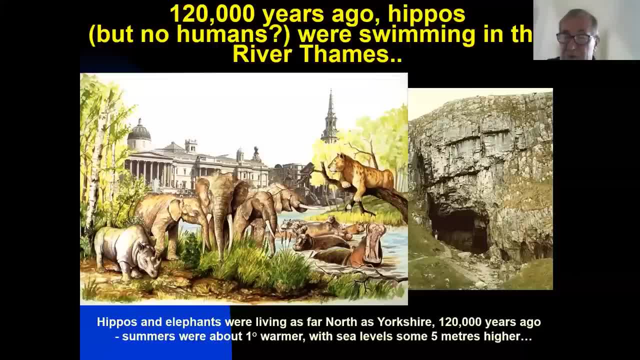 The hippos are even found in caves up in Yorkshire. So this was a time when Britain was warmer than the present day- warmer summers, milder winters- And the sea level at times was some 5 meters higher, And that means it looks like Britain had become an island at this time. 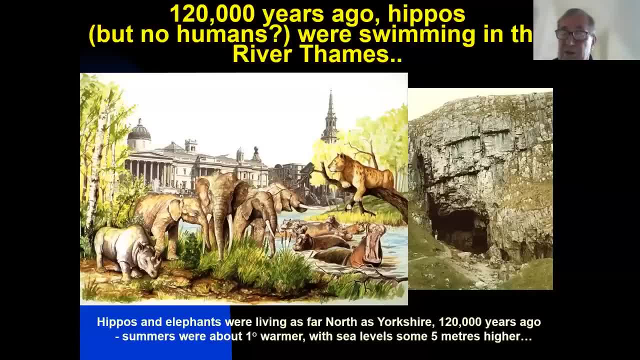 And what's interesting is we have no archaeology associated with this fauna, what we can call the Trafalgar Square fauna, which correlates with Marine Ice State 5e, the warmest part of the last interglacial. So there's not a single fauna that we can call the Trafalgar Square fauna which correlates. 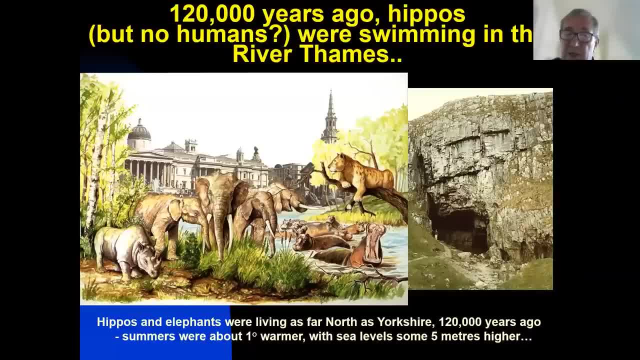 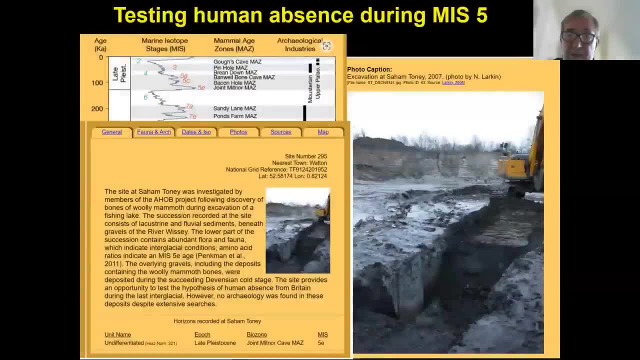 with marine ice stage 5e, the warmest part of the last interglacial single cut mark bone. amongst these assemblages there's not a single artifact reliably associated with this. Trafalgar Square fauna And Ahab actually tested this idea because of course, it's possible. 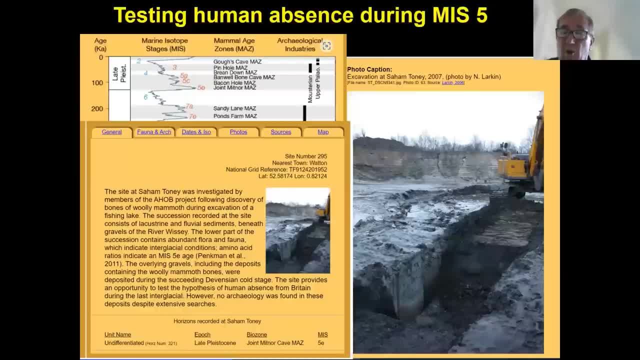 humans were there and we didn't find the evidence. so we went back to old collections and looked for cut mark bones and we actually conducted a major excavation of a site called Sam Tony, which had parts of stage five represented, excavated a lot of material, a lot of fauna material. we didn't find. 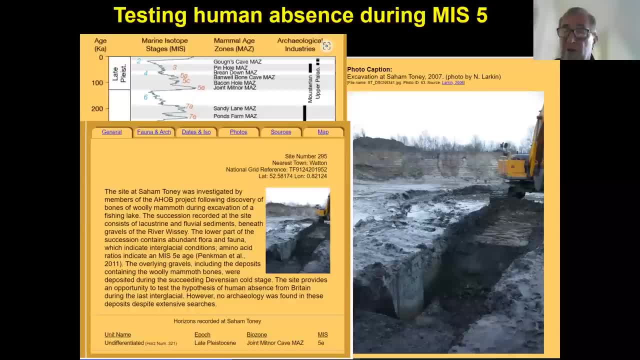 a single cut mark bone from this site. we didn't find a single artifact from these very extensive excavations. So, as far as we're concerned, this idea of human absence, of Britain being an island where fauna got across but not the Neanderthals for MIS 5e at the moment, this model stands for us. 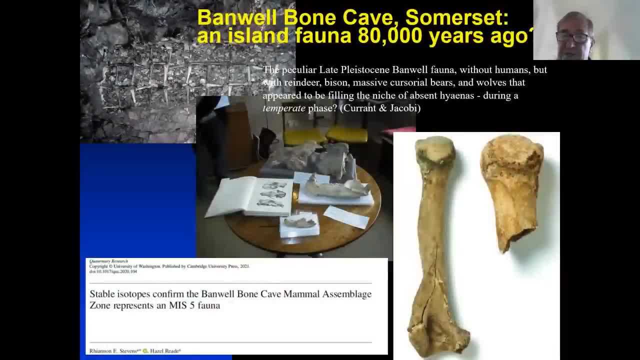 And, remarkably, as stage five continues, marine ice at stage five continues. we still don't seem to see clear evidence of humans. even though sea level was rising and falling, there's still not clear artifact or cut mark evidence from marine ice at stage five. And there's this remarkable fauna. 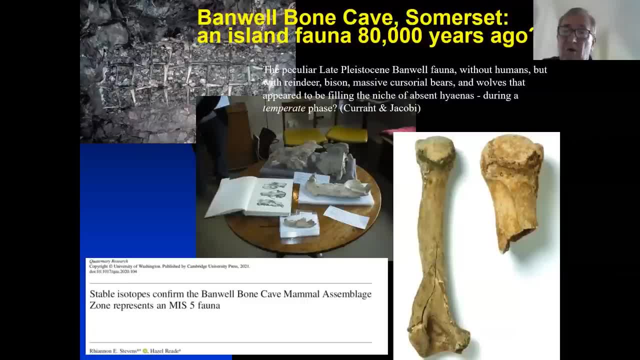 called the Bamor fauna, where you've got apparent cold, represented animals like reindeer and bison, huge bears, probably bigger even than polar bears, Wolves that seem to have been crunching bones like hyenas, and yet they seem to be in a temperate phase And Andy Curran and Roger Jacoby proposed very boldly that this was a fauna that had come. 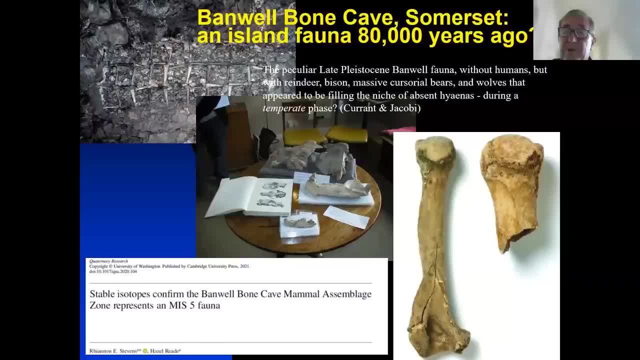 into Britain during MIS 5b, about maybe 90,000 years ago, and had then become isolated in Britain by the subsequent sea level rise. So there's a rapid sea level rise in marine ice at stage 5a and this fauna was trapped in Britain. 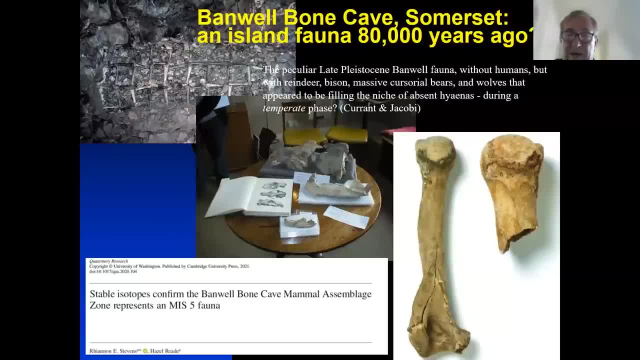 Even though it was a cold fauna. I must admit I had my doubts. although my name was on one of the papers talking about this, I had my doubts about it, but recent isotope work by Rhiannon Stevens and Hazel Reid seems to confirm this idea that the Bamor bone cave fauna is indeed a cold fauna. 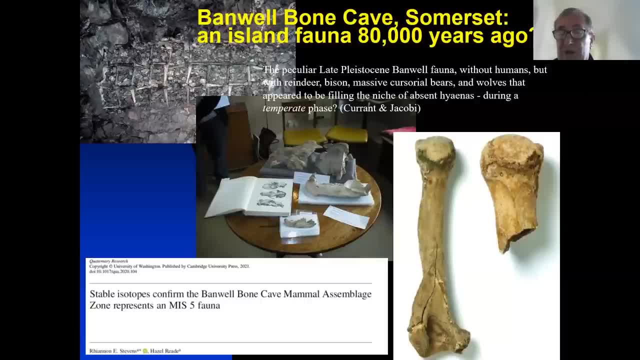 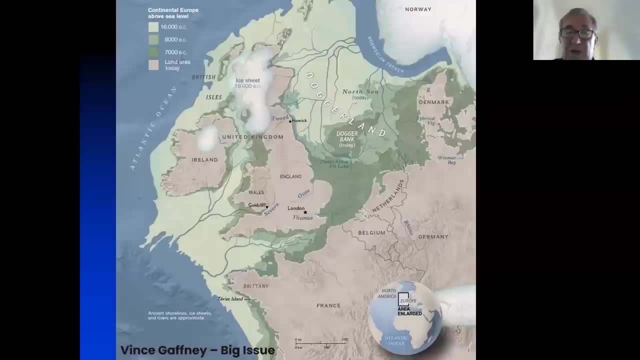 living in a relatively warm environment. So, curiously, still no humans apparently present in the later parts of marine ice at stage five about 80,000 years ago, And now though, Doggerland seems to come increasingly into the picture, So where the Norse is today. we had a very extensive build-up of sediments and the development of the huge land mass that effectively doubled the size of Britain and running through right across to Denmark, as you can see in this excellent reconstruction from Vince Gaffney. 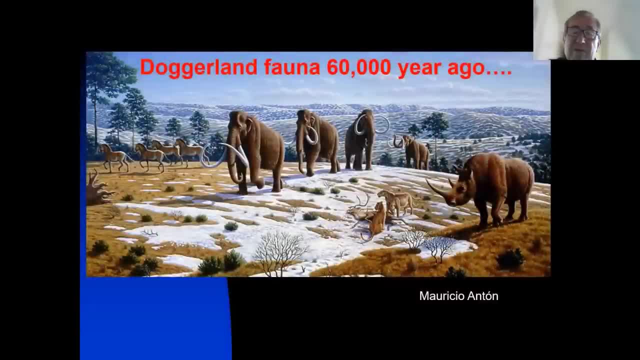 And so these are the kinds of animals that were roaming around on Doggerland about 60,000 years ago. And this is an example of the kind of animals that were roaming around on Doggerland about 60,000 years ago. And this is an example of the kind of animals that were roaming around on Doggerland about 60,000 years ago. 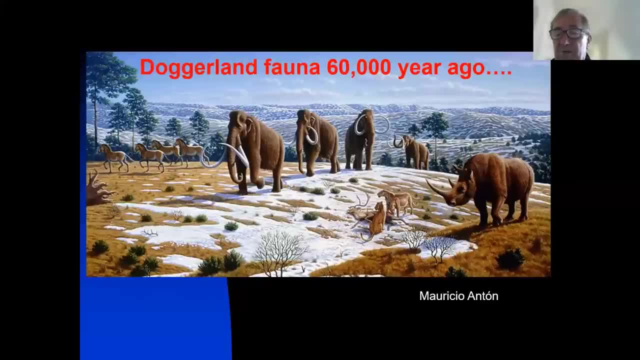 And this is an example of the kind of animals that were roaming around on Doggerland about 60,000 years ago. We've got remains of mammoth, woolly, rhino, lions, reindeer horse, and these remains are found on the. 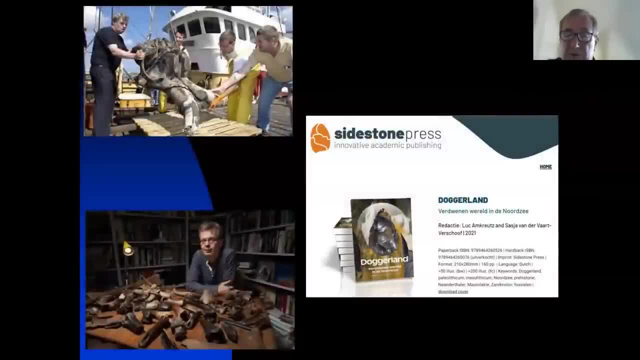 floor of the North Sea and they're regularly dredged up by fishermen. So you can see plenty of evidence in museums and there are books written about it. If you look on eBay, you can even find fossils from the North Sea. although I'm not in favour of the 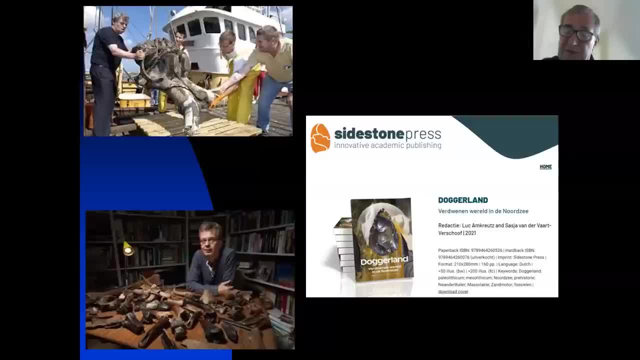 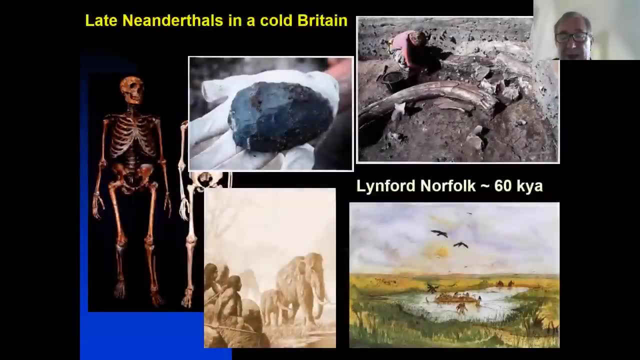 sale of those fossils in a commercial way. I think they ideally should be in museums. But Neanderthals were back in Britain finally by 60,000 years ago. We picked them up at the site of Linford in York, And so there we've got the remains of about 10 mammoths, partial skeletons of mammoths. 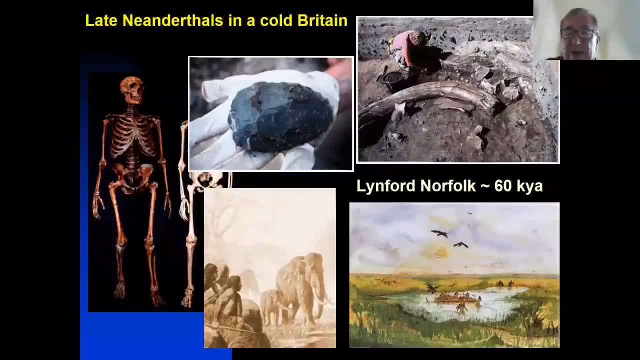 You can see a mammoth tusk there on the top right, and in amongst these mammoths are some of these beautifully made small hand axes which match with ones made by Neanderthals at this time in continental Europe. So it's possible, of course, that the Neanderthals were actually hunting these mammoths, but 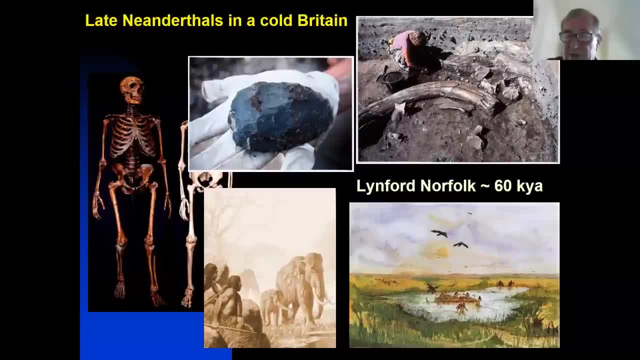 I think it's equally possible, as the reconstruction on the bottom right suggests, that Neanderthals might even have been crossing across to Britain from Europe across Doggerland, coming into what's now Norfolk 60,000 years ago as it warmed up in the spring. 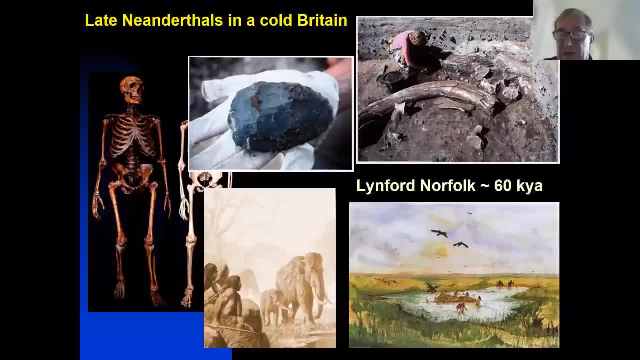 and perhaps even finding dead mammoths defrosting out of glacial lakes in the spring melts, And I'm sure they wouldn't have turned their noses up to defrosting mammoth meat. So that's Linford about 60,000 years ago, and Neanderthals are back in Britain. 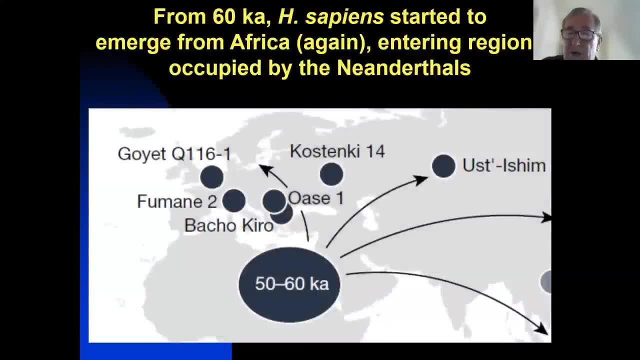 And then, of course, we move on to this time around 60,000 years ago, when geneticists estimate that there was a major dispersal of Homo sapiens from Africa. There had been earlier ones, but there's a major one, the one that really gave rise to the genetic variation we have outside of Africa today. 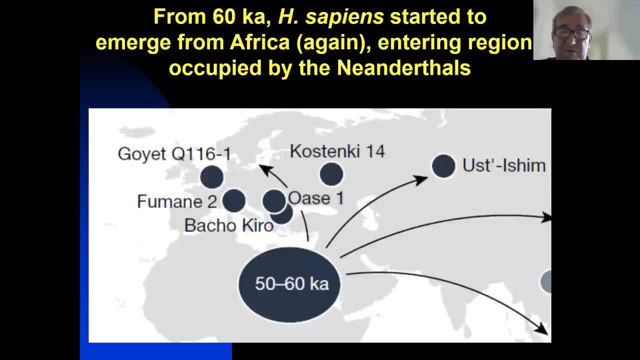 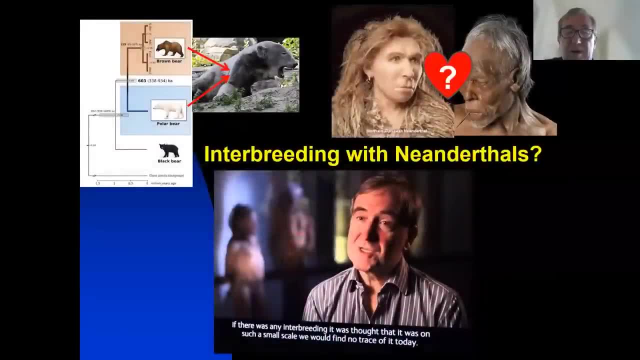 And this obviously was bringing people into the territory of the Neanderthals. So that thorny question of interbreeding that we argued about for a long time and my view was: well, I was aware that closely related mammal species could hybridize, such as 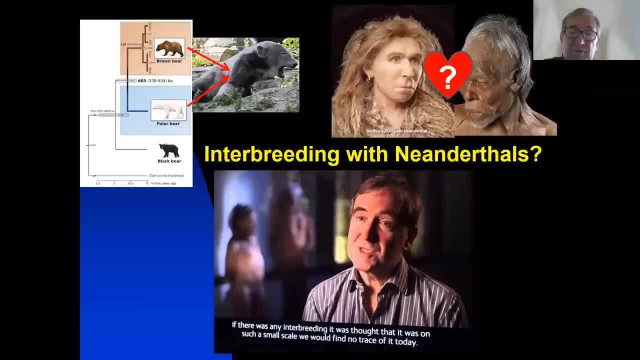 brown bears and polar bears, separating on the same sort of time scale as us, and Neanderthals, baboons, chappals and wolves. they can hybridize. And so I thought that even if we were a different species morphologically, as I believe my view was until recently, if there was any interbreeding it was on. 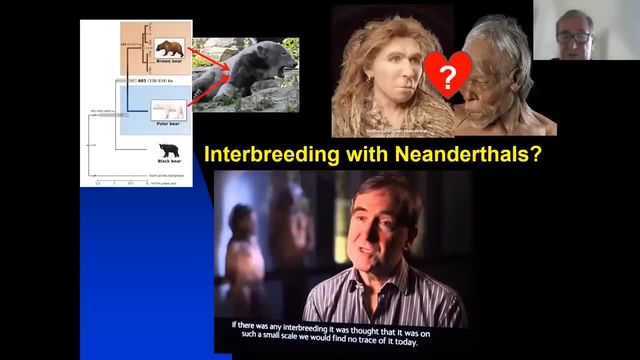 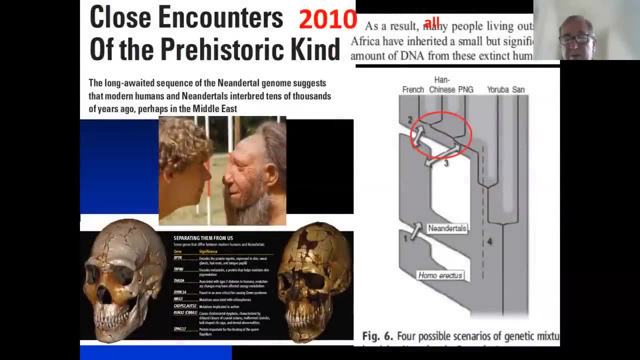 such a small scale, we would not find no trace of it today And of course, I was wrong about that, Because in 2010, we start to get the publication of high quality Neanderthal genomes and they showed clearly that they had been interbreeding. So, as it says here from Journal of Science: The long awaited sequence of the Neanderthal genome suggests that modern humans and Neanderthals interbred tens of thousands of years ago, perhaps in the Middle East. As a result- and I've corrected it pretty well- everyone living outside of Africa has inherited a small but significant amount of DNA. 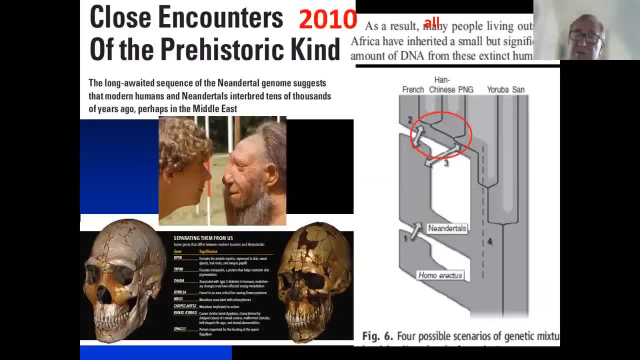 from these extinct humans. So the hypothesis is that there was interbreeding. as Homo sapiens came out of Africa into Western Asia, they met Neanderthals. there was some interbreeding. And as they spread out further into the rest of Eurasia and eventually Southeast Asia and the 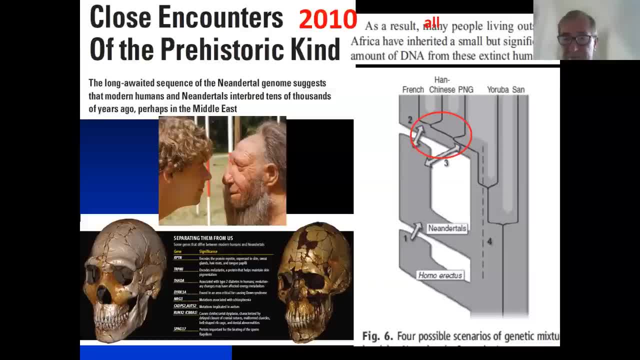 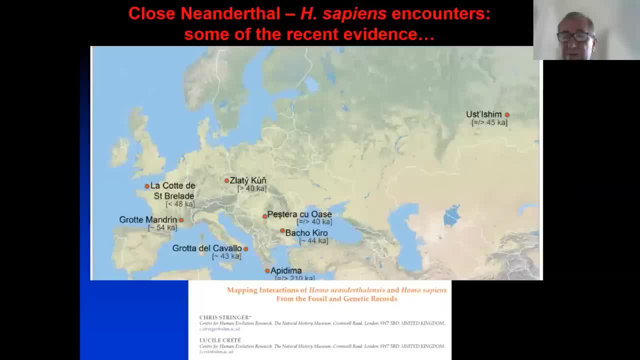 Americas. they took that bit of Neanderthal DNA with them. So I read a review paper a few months ago with Lucille Crette about this interesting period of time, this interesting period of overlap in Europe, and there's more information in there about this period and the wonderful. 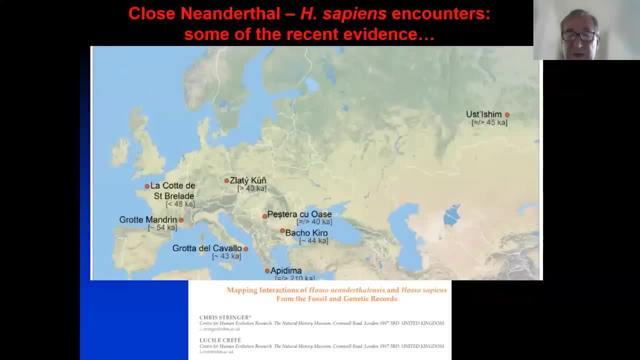 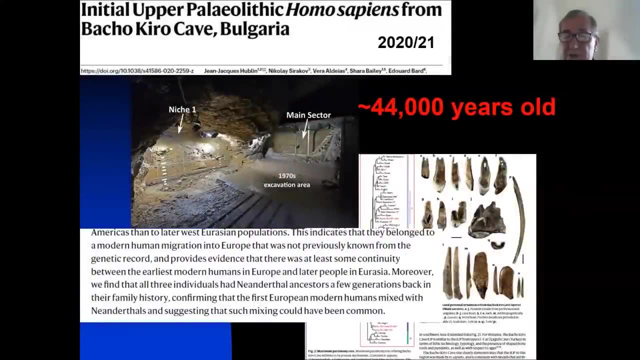 data that's coming through, both from fossils and from the DNA data. So, for example, the wonderful site of Pachukiro about 44,000 years ago, fragmentary Homo sapiens fossils with quite rich material culture evidence excavated by Georgiak-Kublan, and. 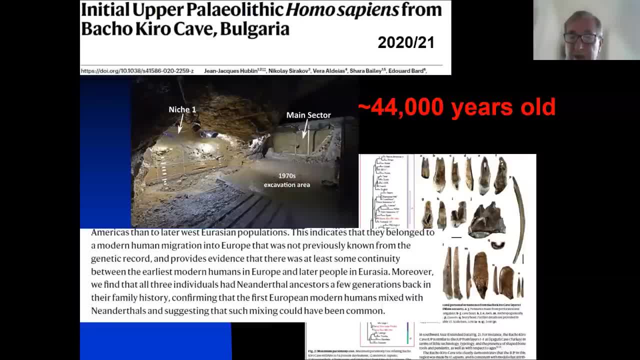 colleagues, And as it says here from the DNA data, this indicates that they belong to a modern human migration into Europe that was not previously known from the genetic record and provides evidence that there was at least some continuity between the earliest modern humans in Europe and later people in Eurasia. Moreover, we find that all three individuals 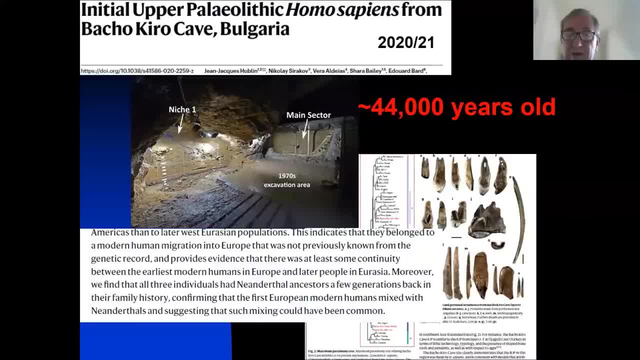 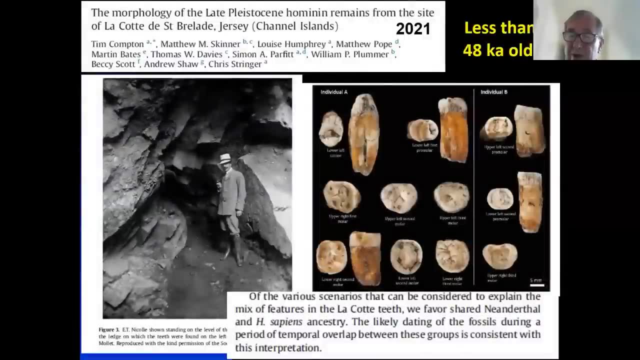 had Neanderthal ancestors a few generations back in their family history, confirming that the first European modern humans mixed with Neanderthals and suggesting that such mixing could have been common. And perhaps we have the same story closer to Britain because we have a series of teeth from 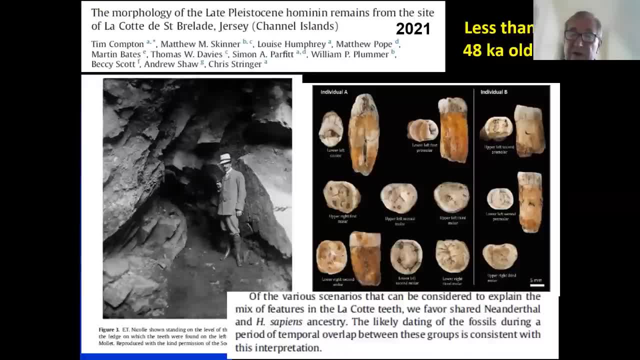 La Côte d'Isambrellade in Jersey, And these teeth were found over 100 years ago and were thought to represent probably a single Neanderthal individual. But I've worked with colleagues like Tim Compton and Matt Skinner in looking at these teeth again, And the remarkable thing is, first of all: 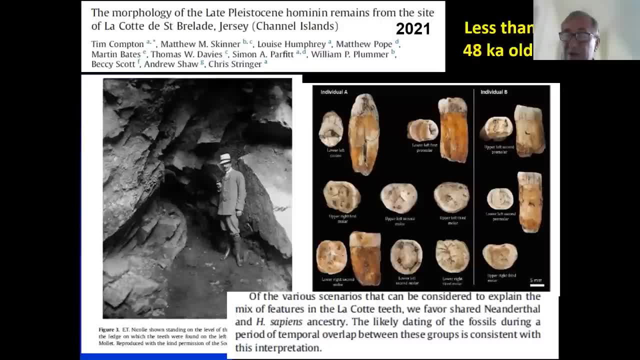 they discovered from their really detailed studies that there were actually two individuals represented in this assemblage and not just one individual. And what was remarkable was, yes, there were Neanderthal features on these teeth, For example, these torodont roots, which are very 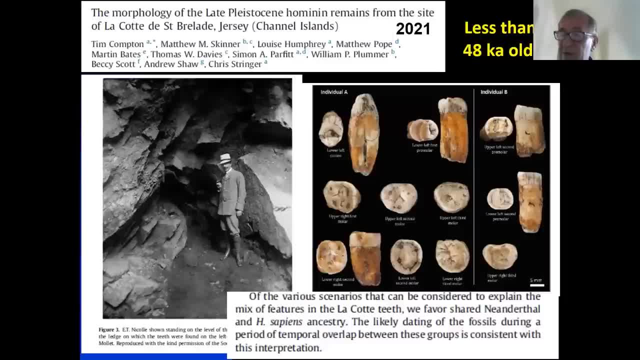 Neanderthal-like, But as you looked at the crowns of the teeth, they look much less like Neanderthals and more like Homo sapiens. So how to account for this? Well, we think these teeth are less than 48,000 years old, And so, as we concluded in this paper in JEG, of the various scenarios that can, 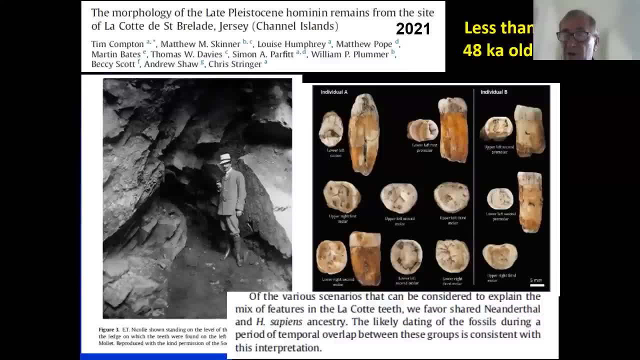 be considered to explain the mix of features in the La Côte teeth. we favour shared Neanderthal and Homo sapiens ancestry. The likely dating of the fossils during the period of temporal overlap between these groups is consistent with this interpretation, So possibly. 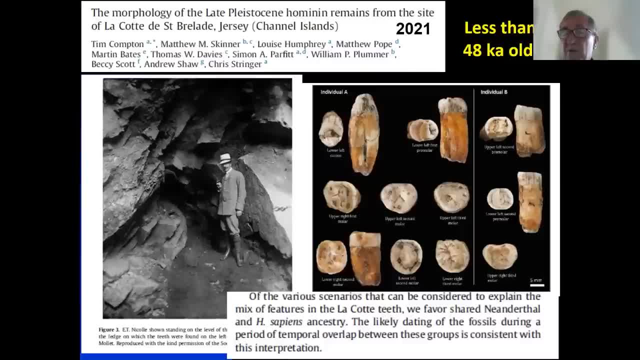 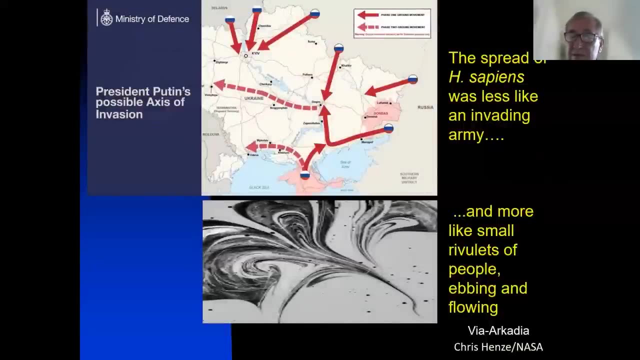 Neanderthals were a population of mixed heritage living on the Channel Islands on Jersey less than 48,000 years ago, And obviously it would be great to get DNA from these teeth And that's something we're looking into at the moment. So how were these events occurring of Neanderthals? 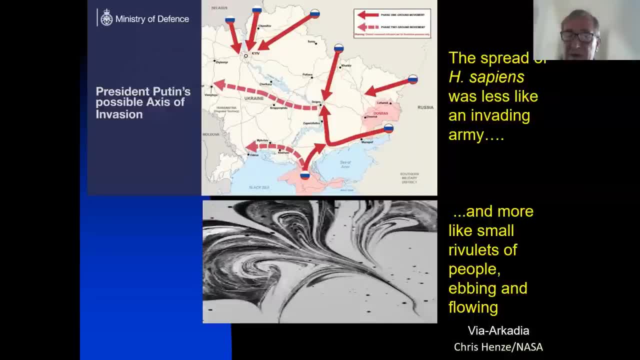 meeting Homo sapiens. Well, at the top, here we've got a reconstruction of President Putin's supposed invasion of the Ukraine. It didn't happen that way, of course, but you can see this invading army supposedly taking over Ukraine. The appearance of Homo sapiens in Europe was 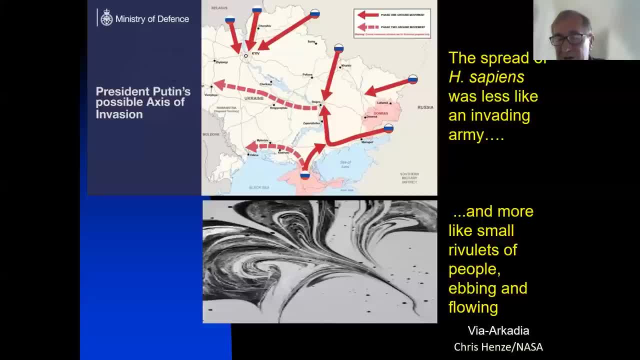 certainly nothing like that, And I think it's much more like the pattern we've got below: small rivulets of people ebbing and flowing at times, small numbers of Homo sapiens and Neanderthals in the landscape at times neither of them there, at times one or other there, at times they're both. there and clearly doing good. So that's what we're looking at here. So we're looking at Neanderthals in the landscape at times. neither of them there at times, one or other there at times. they're both there and clearly doing good. 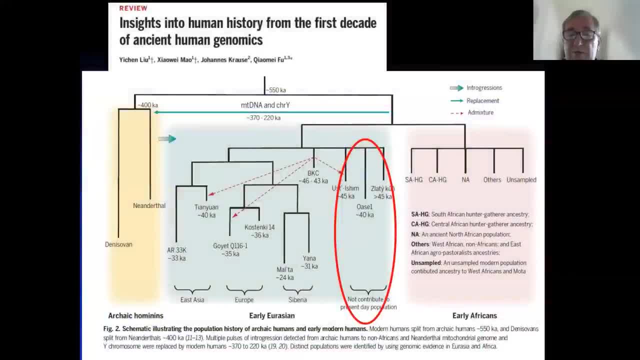 And what's interesting, from the genetic data- and this is the paper by Liu and colleagues- it seems that some of these European populations did give rise to descendant populations in Europe and over in the Far East, but others seem to be in a sense dead ends. They seem to be lost. 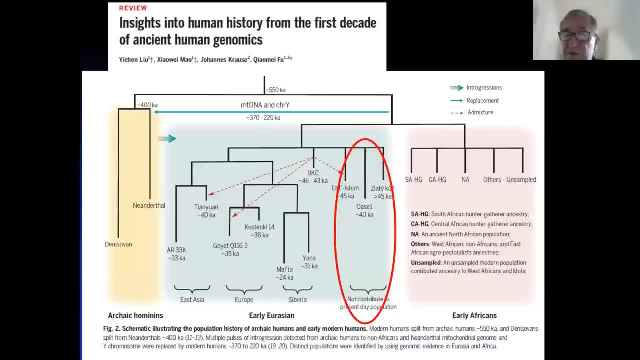 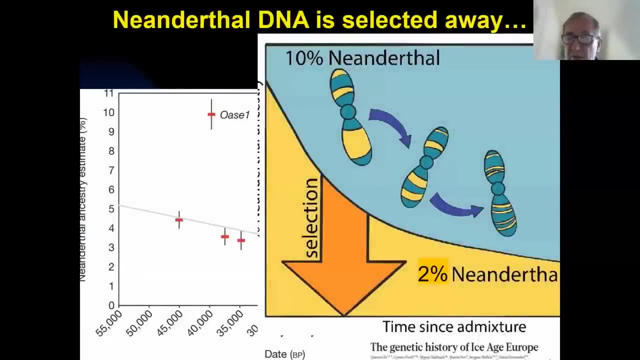 lineages of Homo sapiens, and that seems to be true for the individual, for Ust-Ishim and Ouase and Zulati-Kun. they may not have surviving lineages, So they represent lost lineages of Homo sapiens, And of course, that Neanderthal DNA was then selected away pretty rapidly. As we get DNA. 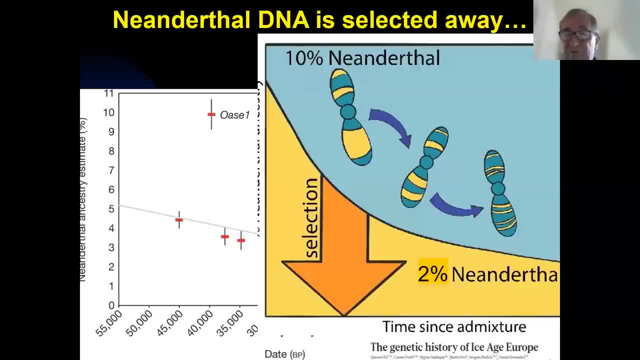 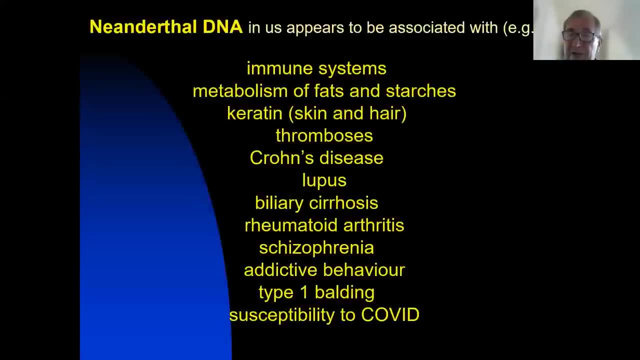 sequences, genome sequences from Homo sapiens. in Europe we find that the amount of DNA is already at an early stage very low, down to the two or 3% that we find today. So there's selection quite rapidly for loss of this Neanderthal DNA, But on the other hand it leaves its mark on us. 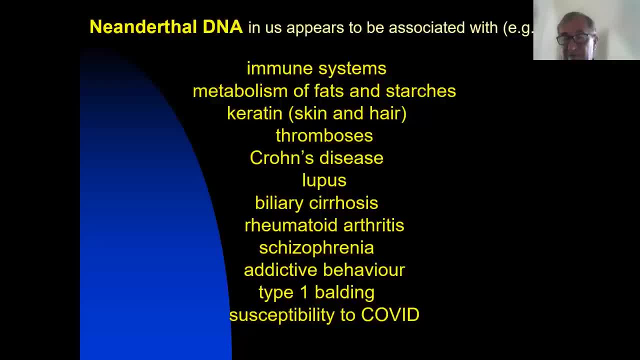 And of course this is really stuff of medical interest- that it seems that this Neanderthal DNA is having an influence today, at least at some level, a small level. So there's a suggestion that there is a correlation between the presence of Neanderthal DNA in particular bits of our 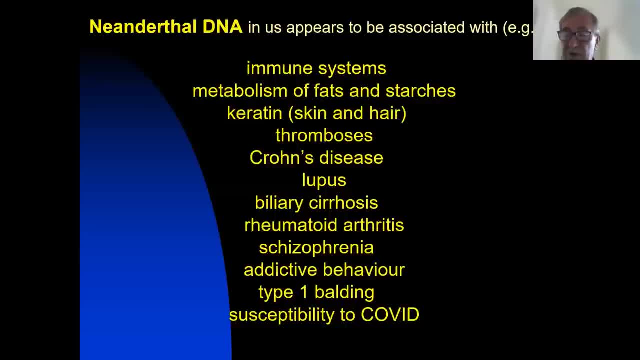 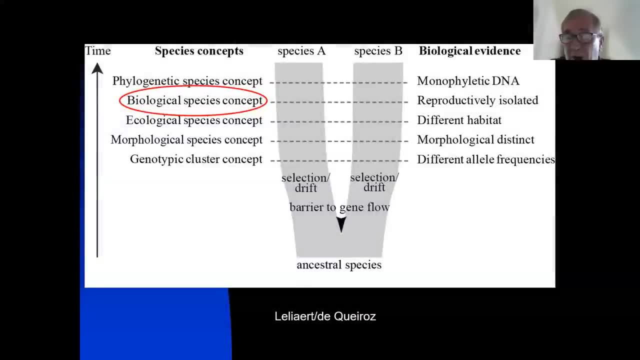 genome and some of these conditions which are found in Homo sapiens today, And if we were interbreeding with Neanderthals? well, are we really a different species to Neanderthals? I think this diagram makes the point very nicely that of course there are. 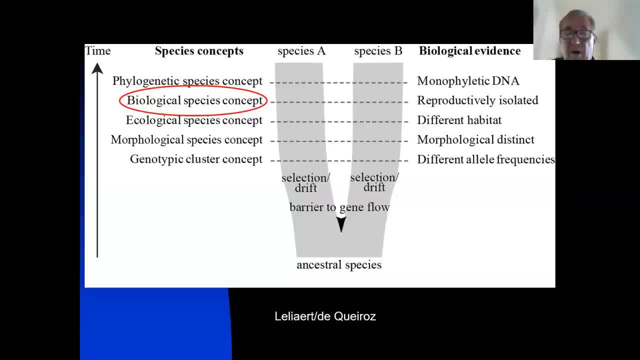 many different species concepts And I certainly think the Neanderthals and us are morphologically different. We're morphologically distinct species. The criteria we use to establish species when we look at other mammals certainly, I think, establish that we are Neanderthals. We're distinct species, But we were not. 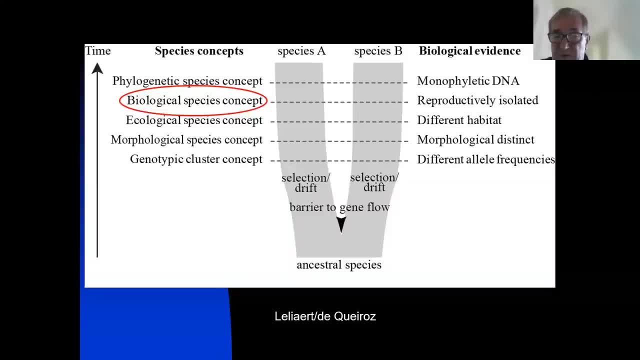 yet biologically distinct species. So the biological species concept is something that applies really some way through the evolution and separation of species. So we and Neanderthals were clearly not distinct enough to yet have reproductive isolation- that characterizes the biological species concept. But we certainly had the morphological differentiation. 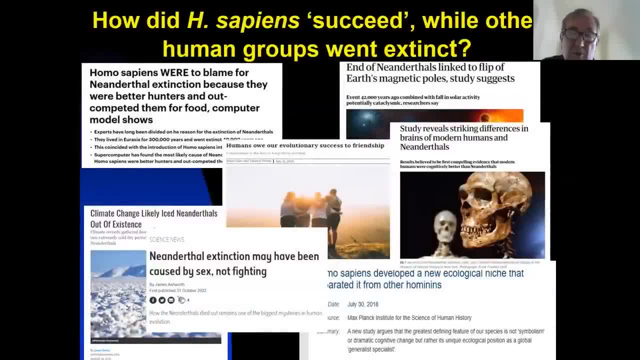 And how did we succeed in, In taking over Europe from the Neanderthals? Well, it was certainly not an overnight thing. It took many thousands of years. And in a sense, the Neanderthals, because, haven't completely disappeared since their DNA or much of it lives on in us today. So there are many different ideas. 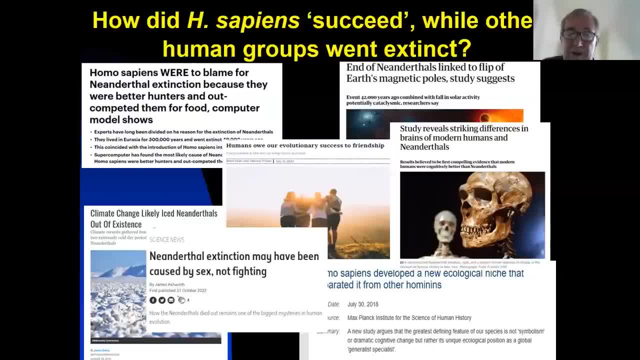 and I haven't got time to discuss them about why we succeeded, But one possibility is that indeed the Neanderthals, who probably were small in number by the time Homo sapiens, came into Europe. the population may have been quite small and perhaps to some extent they were actually. 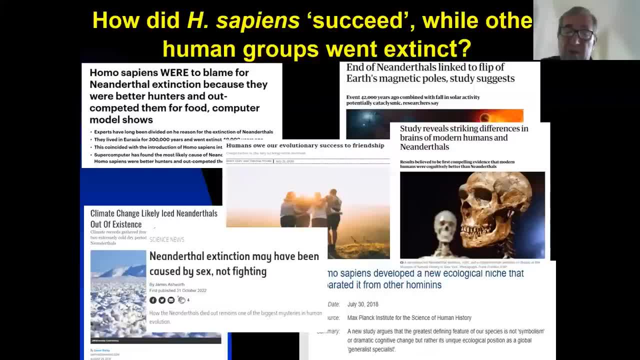 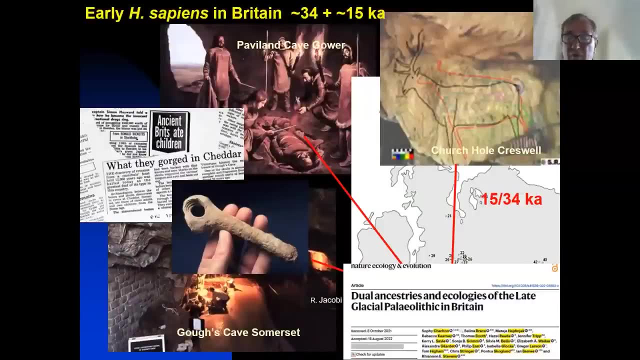 absorbed into the Homo sapiens populations. So extinction by absorption might be a possible model for some of these Neanderthals. And then, getting back to the British story, the Neanderthals we think were in Britain until about 45,000 years ago, And then we have the presence of what are often as transitional. 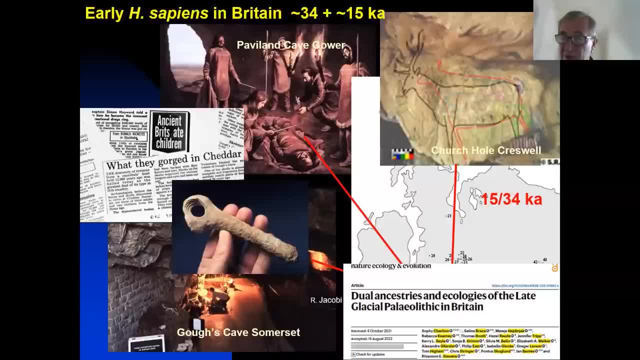 industries, industries, And we don't know who made those. But when we get to about 35,000 years ago, we certainly have Homo sapiens present. at Pavillon Cave in Gower, A man was buried, associated with ivory artifacts, about 34,000 years ago And this is associated with an early part of the. 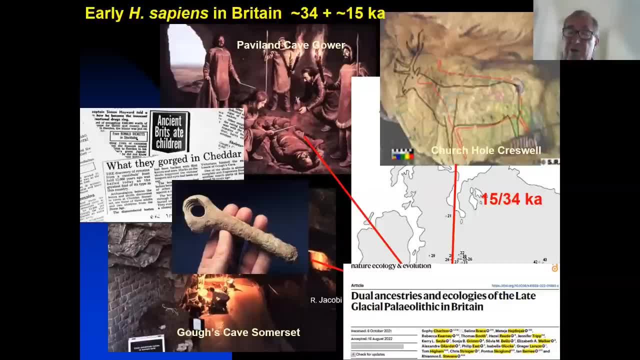 Gravettian culture. There was an Aurignacian occupation of Britain, but we don't have any reliable fossils. There is the maxilla from Kent's Cavern, which Tom and I were involved in studying publishing more than 10 years ago. That seems to be over 40,000 years old. 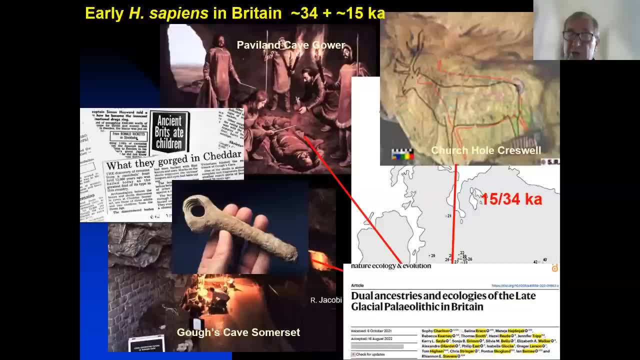 It's a Homo sapiens, but we can't tell its archaeological association. Then we have the peak of the last glaciation. Britain seems to be completely depopulated And then people come back again about 15,000 years ago. We find evidence of their artwork on engravings on the walls. 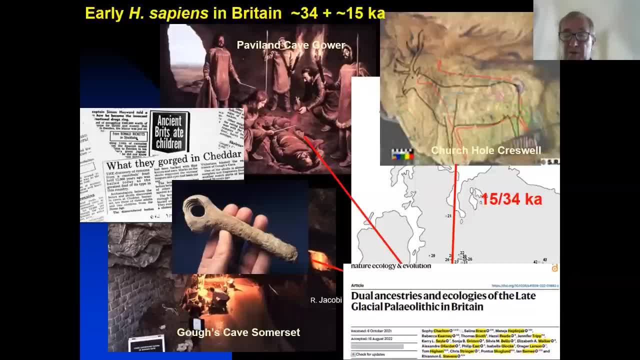 in church And we find evidence of their behavior at Goff's Cave in Somerset, These beautiful so-called batons made out of reindeer, antler and even a bit of cannibalism. going on about 15,000 years ago in Somerset. And now really it's time to end the story and summarize it So. 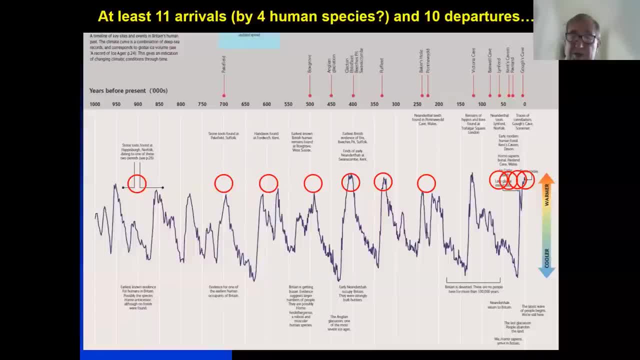 we've had a whistle-stop tour of about 900,000 years And we can summarize it by this diagram from the book I wrote with Rob Guinness. We've written one million years of the human story And, looking at the big picture, we can see. 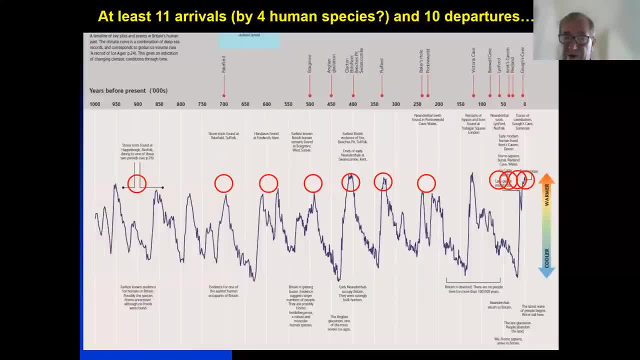 probably a dozen different occupations of Britain through this 900,000 year period And 11 of those disappeared And we're in that last phase now. So we have an occupation in nearly all of these interglacial peaks. It's quite possible there are more of them. We don't have them mapped. 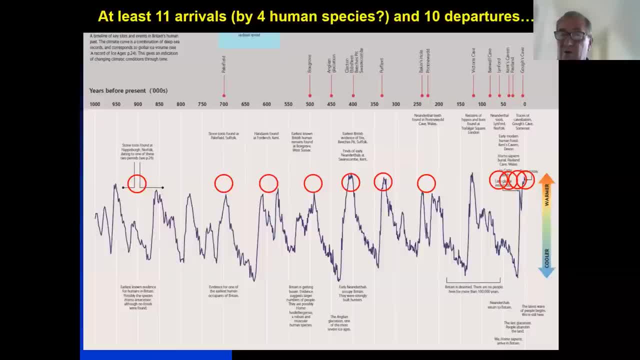 But of course that peak at about 120,000 years ago. we can see that there are about 120,000 years ago on the right there stands out at the moment as uniquely showing a human absence during a later plasticine interglacial. So that's the big story of comings and goings that Britain was populated. 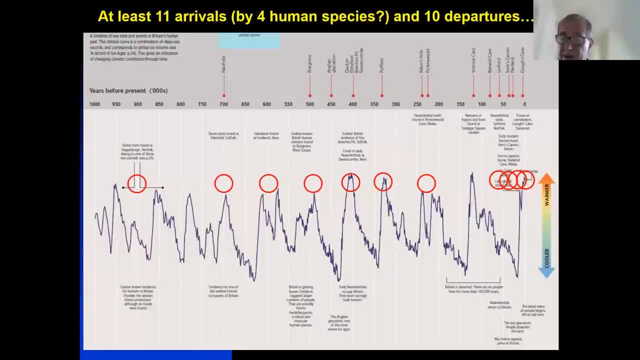 and colonized over and over again. But when the bad weather came, those populations either got out of Britain or they perish completely. And that's the fate of these earlier populations, probably at least four-spot. But that's the big story of the coming and goings and goings And that's the fate of these earlier populations, probably at least four-spot. 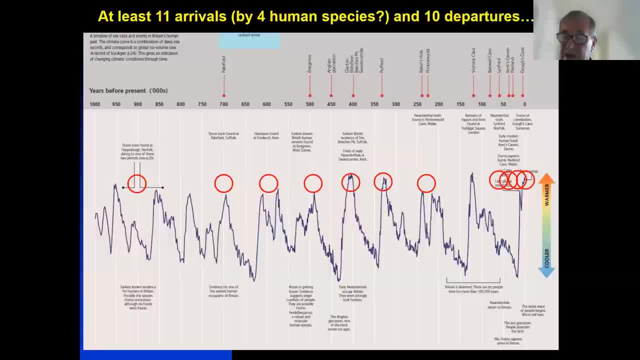 And that's the fate of these earlier populations, probably at least four-spot. And that's the fate of these earlier populations, probably at least four-spot. Homo sapiens. at the end, the Neanderthals, perhaps Homo heidelbergensis. 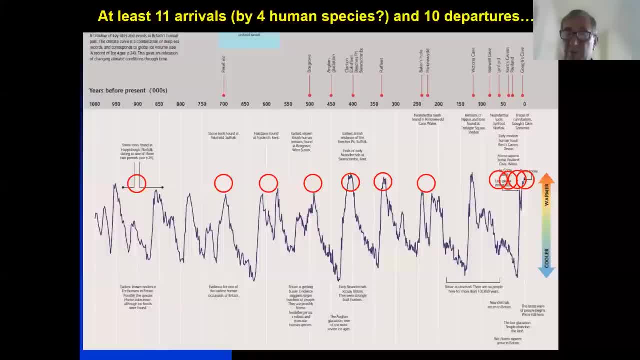 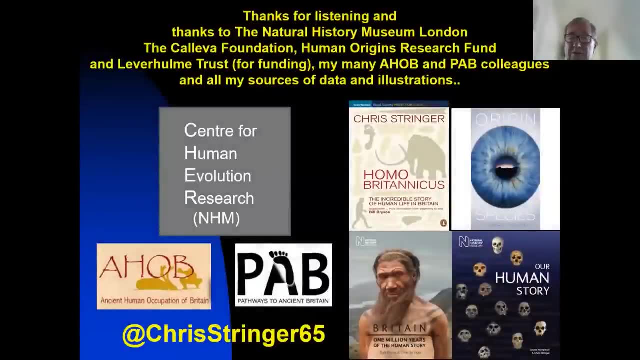 perhaps Homo antisessel, But for those earlier records we need better fossil evidence to establish that. So I'll stop now and just thank everyone who took part in the AHOB projects and now in the ongoing Pathways to Ancient Britain project. All of the work involved, all of the